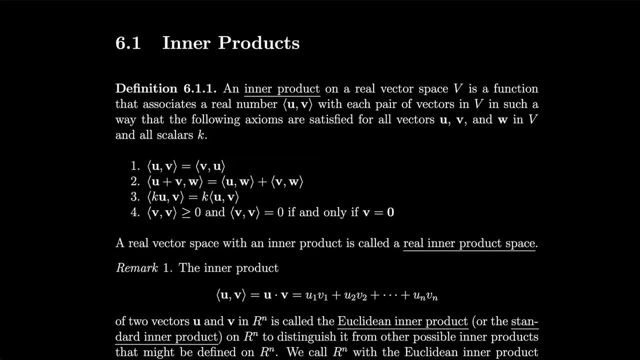 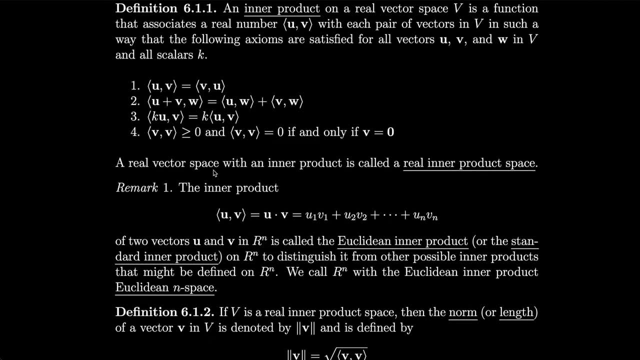 inner product space. So we have a vector space and it also supports these four axioms, then it's an inner product space. The inner product uv, equal to the dot product u, dot v, which, remember, is defined by just multiplying each of the corresponding components and adding them up of two vectors, u and v. in Rn is called the. 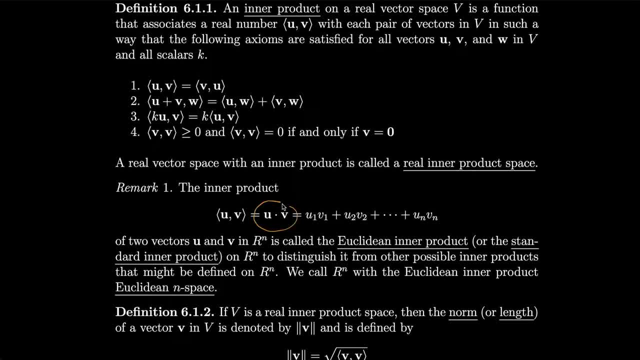 Euclidean inner product. So in other words, the dot product we already did is a special example of a one type of inner product called the Euclidean inner product. So that means we're going to be looking at other inner products so you could think of it as alternatives to the dot. 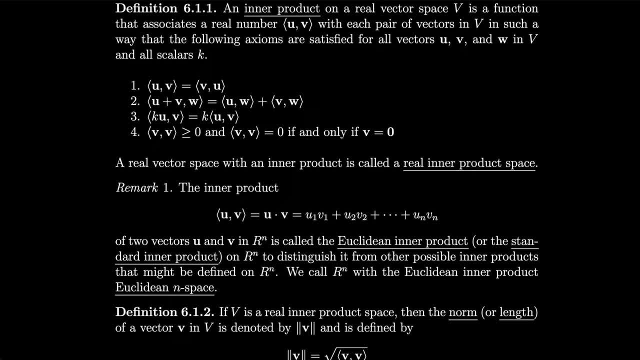 product. This is also called the standard inner product. on Rn, to distinguish it from other possible inner products that might be defined in Rn, We call Rn with the Euclidean inner product Euclidean n space. If v is a real inner product space, then the norm or length of a vector 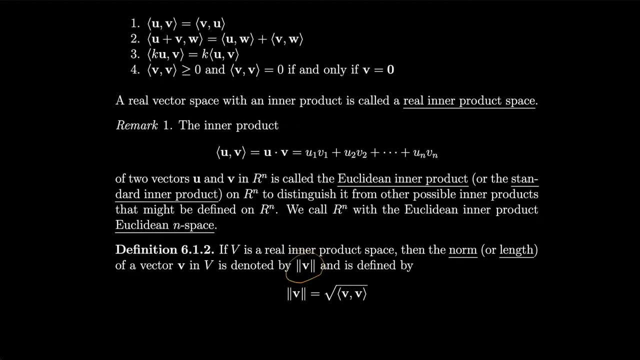 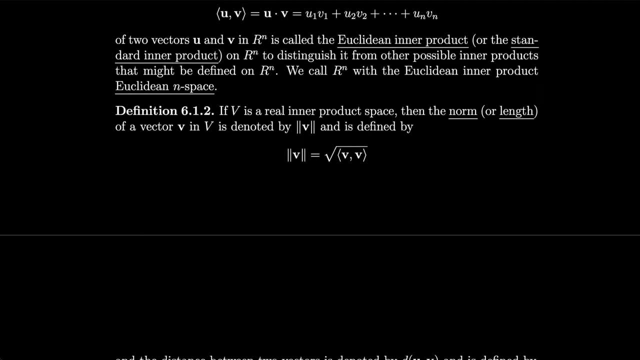 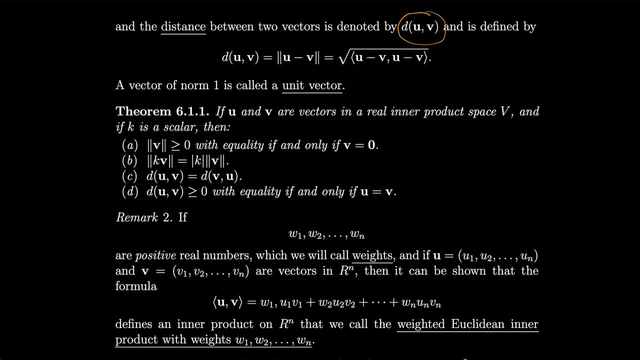 in v is denoted by norm of v, and it is defined by the square root of the inner product of the vector with itself. The distance between two vectors is denoted by duv, and it is defined by the norm of the difference between the two vectors. 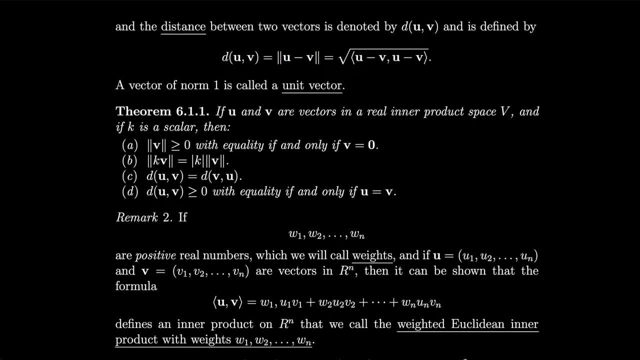 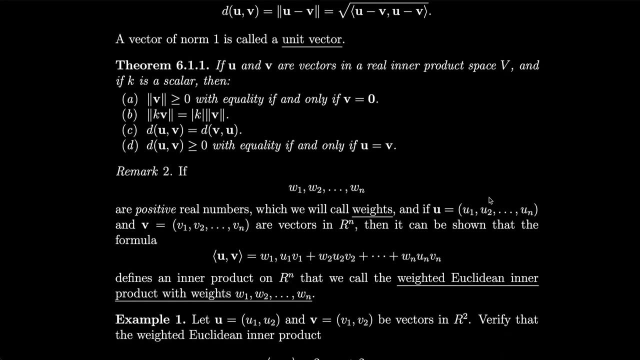 So what we're basically saying is take the inner product of u-v with u-v, take the square root of that and that's the distance between two vectors. A vector of norm 1 is called a unit vector. So next up, if u and v are vectors in a real inner product space- v- and if k is a scalar, 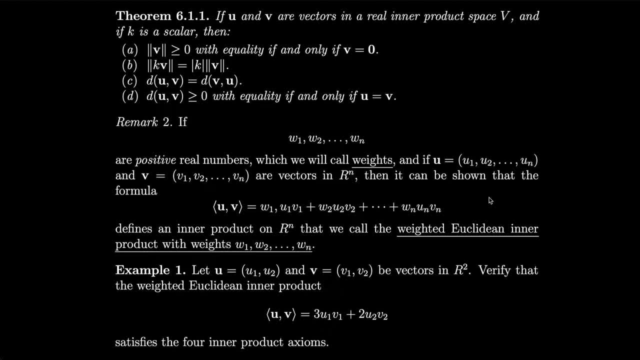 then the length of v is greater than, or equal to, 0, when it equals 0,. if it only is a scalar, then the length of v is greater than or equal to, 0, when it equals 0,. if it, if v is a zero vector, We can pull out the scalar. Basically, these follow from the properties of the. 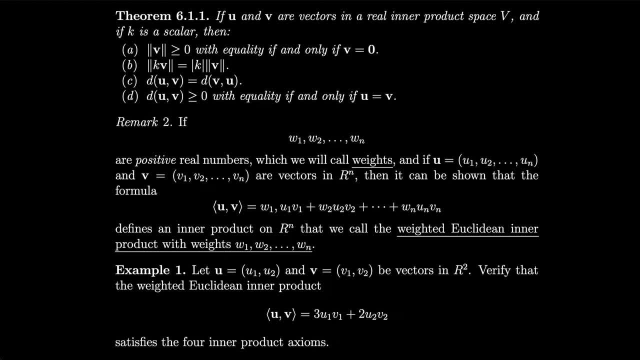 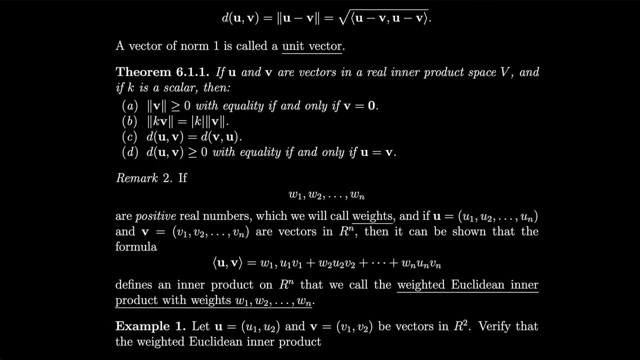 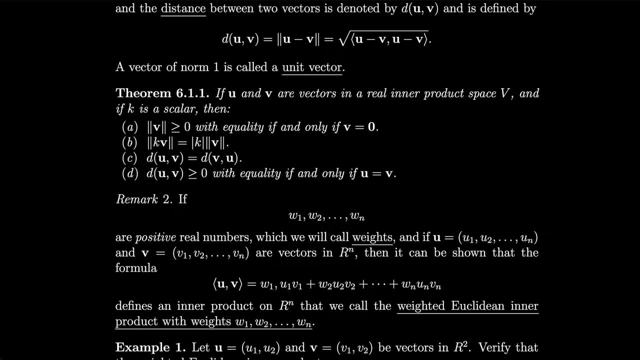 inner product. Since you can pull out scalars from inner products. you can pull out the scalar from the length. The distance between u and v has to be equal to the distance between v and u. That should make sense from the definition, since the inner product of a scaled vector is the same. 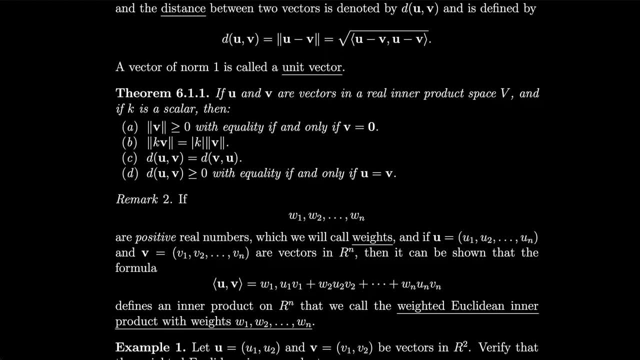 as pulling out the scalar. So that means that if I look at u minus v, then that would be the same as looking at minus v minus u. In other words, if I were to switch this and do v minus u, then that would be the square root of v minus u. Oops, I forgot. 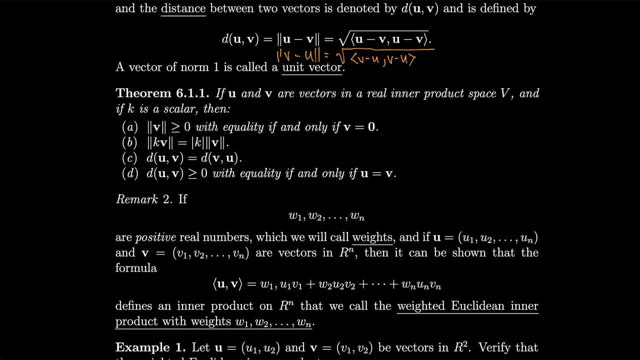 v minus u. but then I could just pull out the minus over here, because this is the same thing as minus times u minus v. So I'd pull out the minus from this one. I'd pull out the minus from this one. The two minuses would cancel. give me a plus, The way I could pull out the minus from. 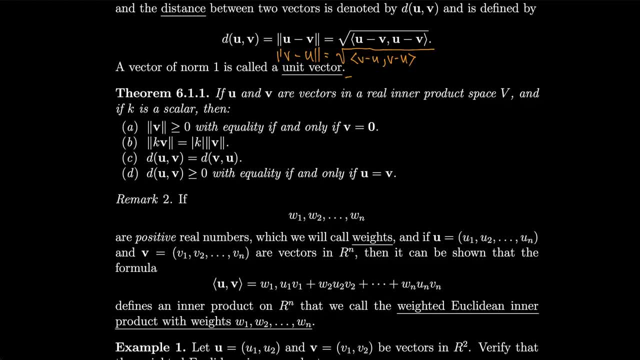 this one is: I could just change the order because, remember, the inner product of u and v is the same as the inner product with v and u. So the two minuses would cancel, because, remember, the inner cancel give us a plus. so this thing would end up being equal to this thing You might want to. 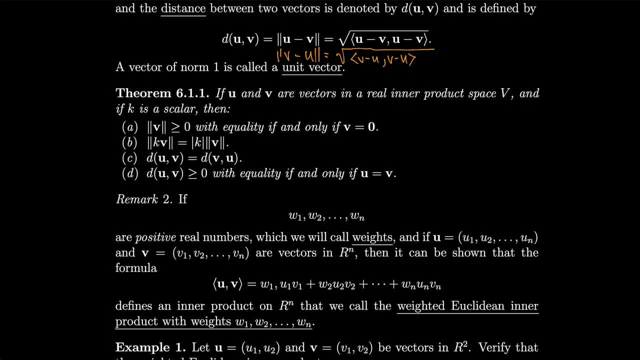 spend some more time to convince yourself. that's true, but in any case it is, and duv is greater than or equal to zero, with equality if, and only if, u is equal to v, If we have w1 through wn, positive real numbers, which we will call weights, and if u equals u1 through un and v equals v1. 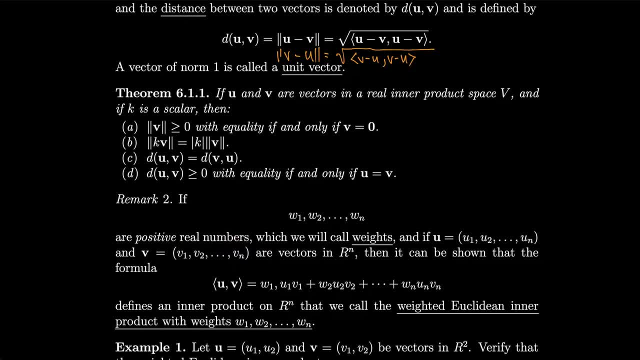 through vn. our vector is in Rn, then it can be shown that the formula uv is equal to w1 times the first u1, v1, first components of u and v. so this is a small typo. it's not supposed to be a. 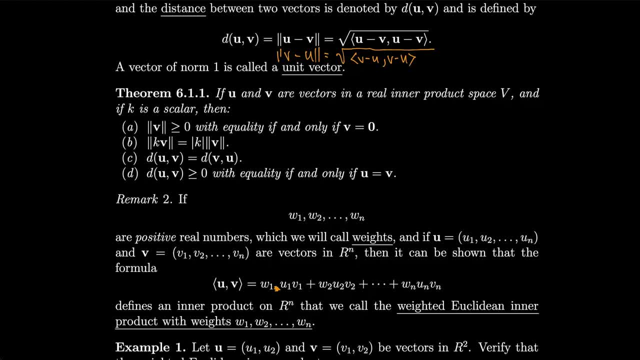 comma there because it's being multiplied, and then w2 multiplies by u2, v2, and so on. wn multiplies through un vn. So that defines an inner product in Rn that we call the weighted Euclidean inner product with weight. 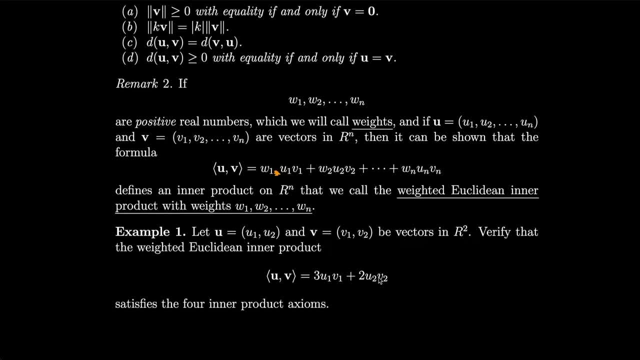 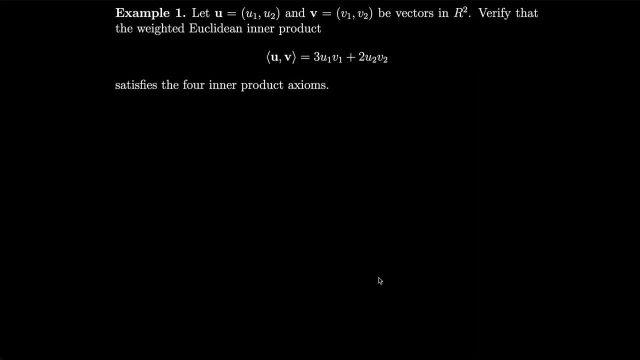 So how about we do an example where we verify that the weighted Euclidean inner product actually does satisfy the four inner product axioms? So we'll check each axiom, kind of like the way that we checked before for things being vector spaces and whatnot. So the first one states that uv. 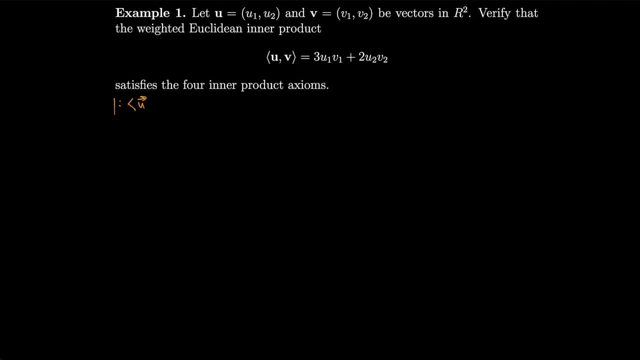 should be vu. so let's look at what the inner product with u and v is. So that's three times u1- v1 plus two times u2- v2, because that's what they told us the inner product should be in this example. So it's just basically a dot product- u1- v1, u2- v2, but it has some weights and the 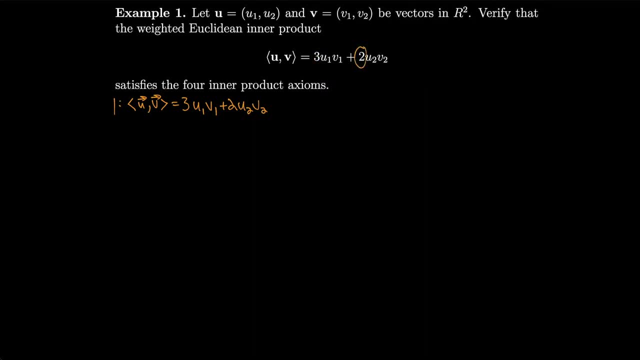 weights don't have to be the same, So in this case, w1 is 3 and w2 is 2.. Well, this is the same thing as if I changed the order right of these two guys, So I could rewrite this. 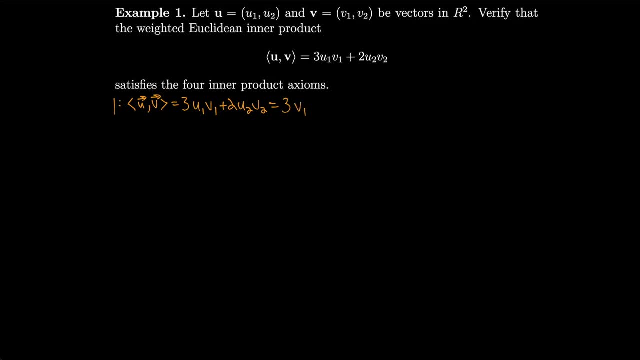 as 3 times v1 times u1 plus 2 times v2, u2, and notice that is just the inner product with v with u, Oops, v with u. Great, so it is symmetric. Let's see if we can spread it out over addition, separate addition out. So let's let w be the vector w1, w2.. 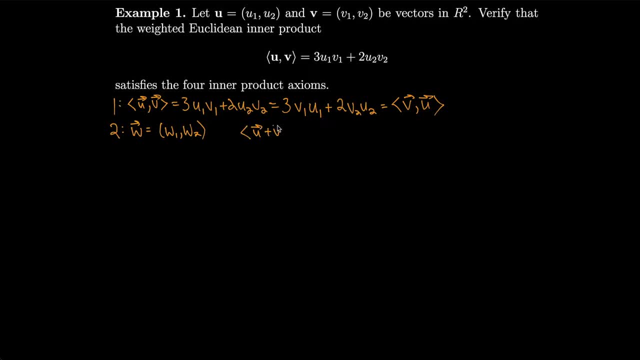 And let's look at what u plus v, inner product with w, should be. So that's three times the first component, which is u1 plus v1.. That's the first component of u1, plus v, And I'll multiply that by the first component w, which is w1.. Add that to 2 times. 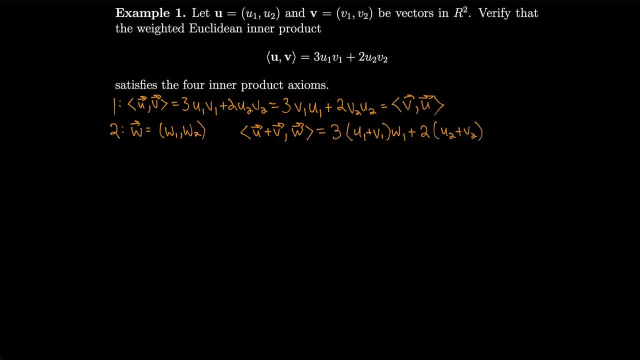 u2 plus v2 times w2.. So I'll multiply out the w's, So I'll get 3 times u1 w1 plus v1 w1 plus 2 times u2 w2 plus v2 w2.. And that equals when I distribute the 3 and the 2, and I'll 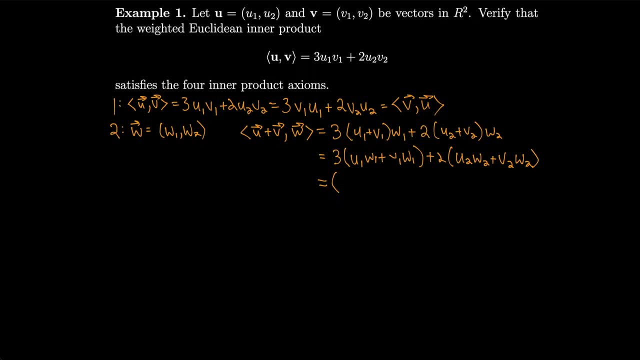 move together the u1 and u2 terms so that it looks like I have a 3 and a 2 in each set. Here I'll show you what I mean: I'll take 3, I'll distribute it and I'll take the 2 and distribute it also And I'll group together the 3u1- w1 with the. 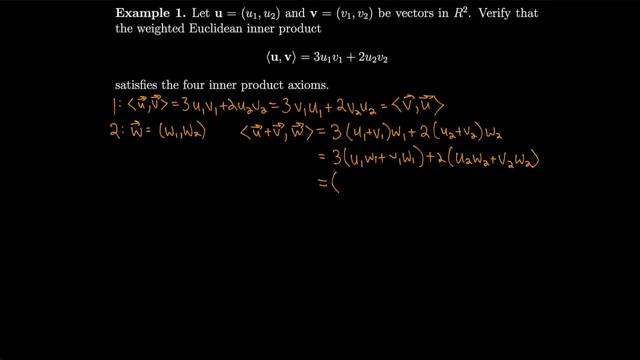 2u2 w2 so that I get an inner product that was defined above. So I'll get 3u1 w1 plus 2 u2 w2, just out of this times. this plus this times this, And then the remaining components will be. 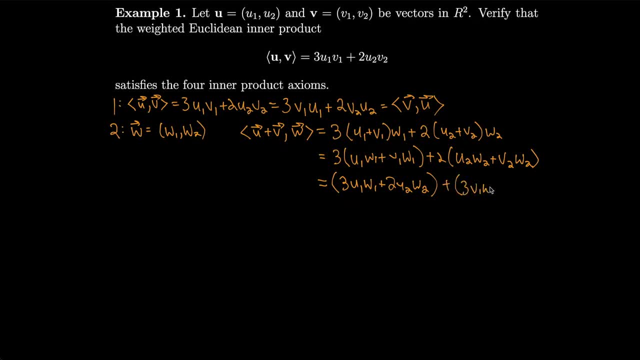 3v1 w1 plus 2v2 w2.. And I wrote it like that because now I can very clearly see that this is an inner product as defined in the example. and this is an inner product as defined in the example. 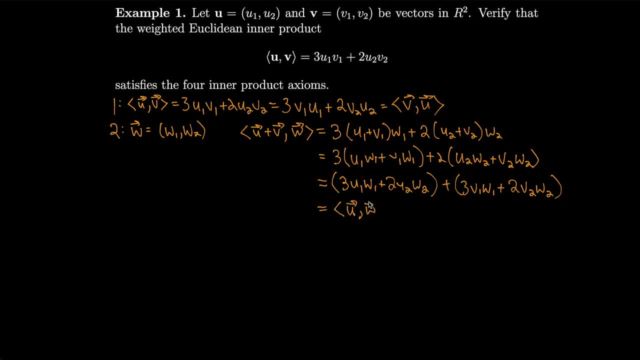 inner product between u and w, and the second one is the inner product defined between v and w. okay, so that's great. so then, this does satisfy the second axiom because it splits over addition. let's look at number three. third axiom was for the constants being able to be pulled out. so 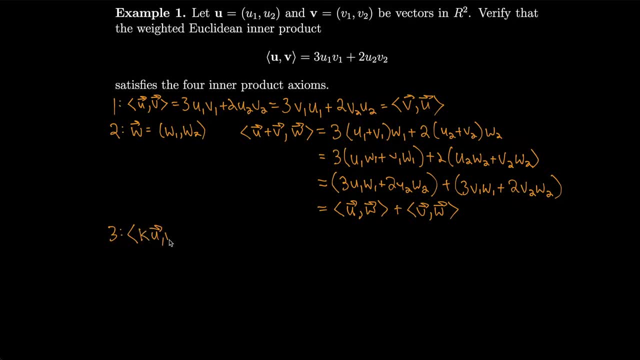 let's see if we could do that k times u- inner product with v. well, that's equal to three times k- u1 times v1 plus two times k- u2 times v2. okay, so how about i factor out k, so i'll get k times three u1 v1 plus two times u2 v2. 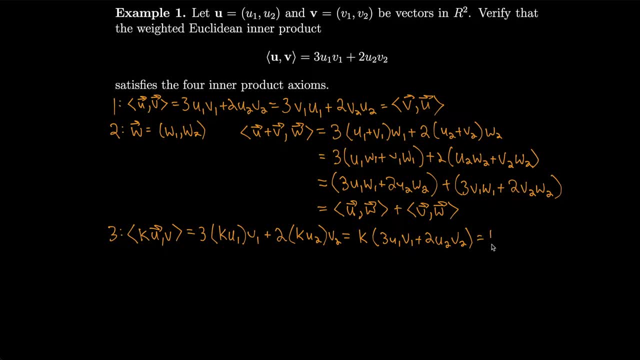 well, that's cool, because that's just k times the inner product with u and v. okay, how about number four? let's look at what happens when we take the inner product of v with v. okay, so that's three times times v1 times v1, plus 2 times v2 times v2, so that's 3 times v1 squared plus 2. 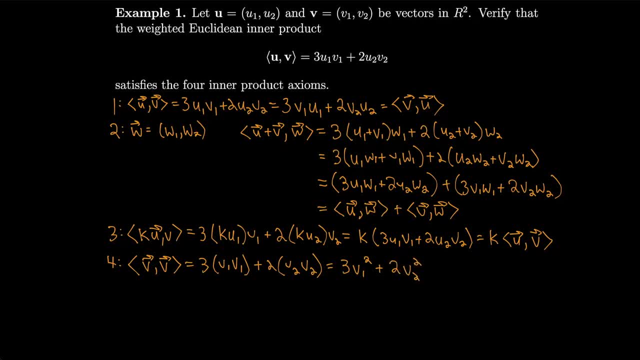 times v2 squared, and because these are both squares, they can't be negative. so this thing will definitely have to be greater than or equal to 0.. Okay, so that means that we have the inner product greater than or equal to 0, but we also 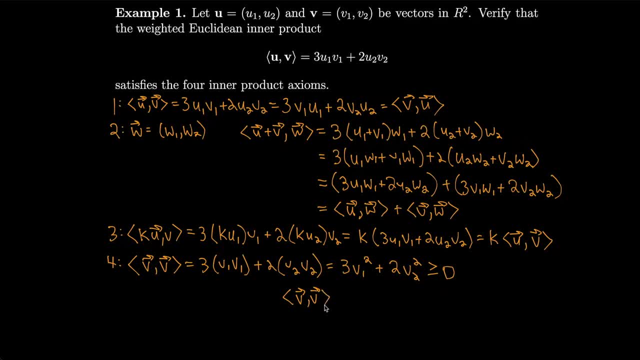 can see that the inner product of v with v will be equal to 0 if, and only if, we have v1 is equal to 0 and v2 is equal to 0. That's the only way to get that equal to 0. So v1 would have to be equal to v2, which would have to be 0, but that's the. 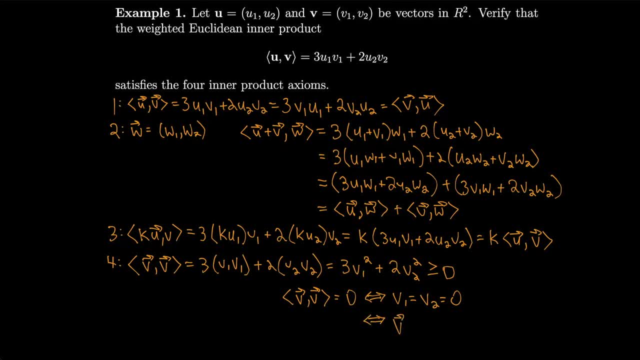 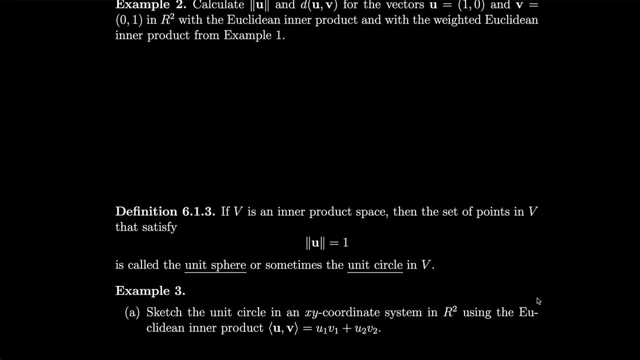 exact same thing as saying that v would have to be the zero vector. Okay, so this inner product actually does satisfy the four inner product axioms. so the weighted Euclidean inner product is an inner product. How about we calculate the length of u and duv for the vectors? 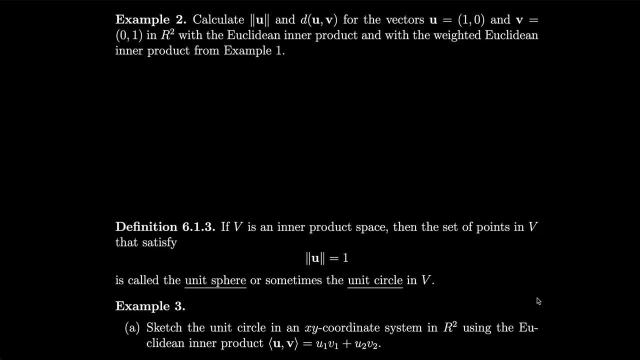 u equals 1, 0 and v equals 0, 1 in R2 with the Euclidean inner product and with the weighted Euclidean inner product from example 1.. So we'll show that we actually do get different lengths and distances depending on what inner product we're using. So it's: 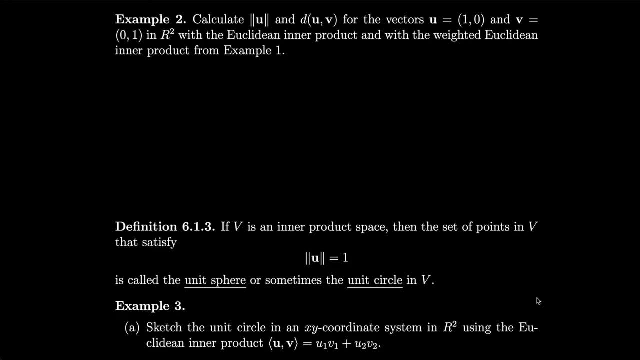 very important to choose the right inner product for the problem or just pay attention to what inner product is stated in the problem. So let's look at the Euclidean one first. So for the Euclidean inner product we have that the length of u or the magnitude of u is equal. 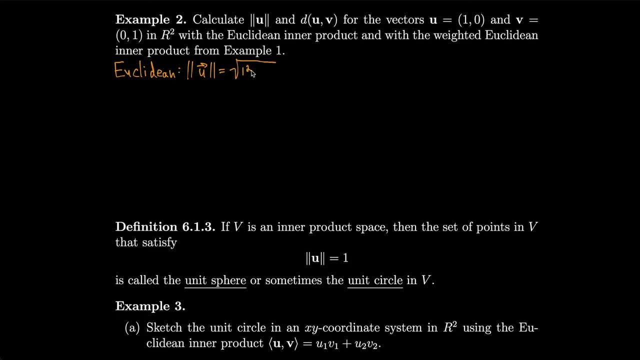 to the square root of 1 squared plus 0 squared, because we're looking at 1, 0 and that's equal to 1.. And how about the distance between u and v? Okay, so that's u minus v, and then we take the length, So that's. 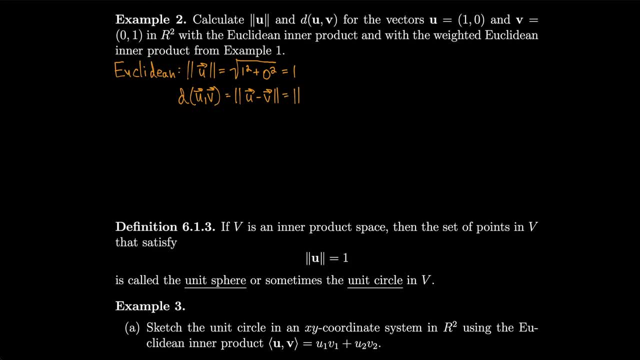 the length of. well, we have 1, 0 minus 0, 1.. So that's 1 minus 1.. And the length of that is just the square root of 1 squared plus minus 1 squared, So that's the square. 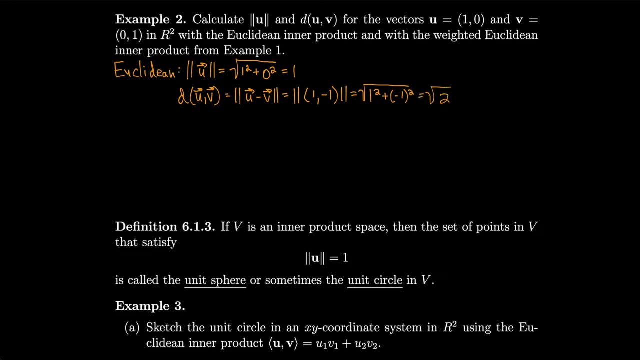 root of 2.. Okay, let's check weighted u Euclidean now, And this is not the general weighted Euclidean. This is specifically the one from the previous example where we had the 3 and the 2. There could have been any constants. 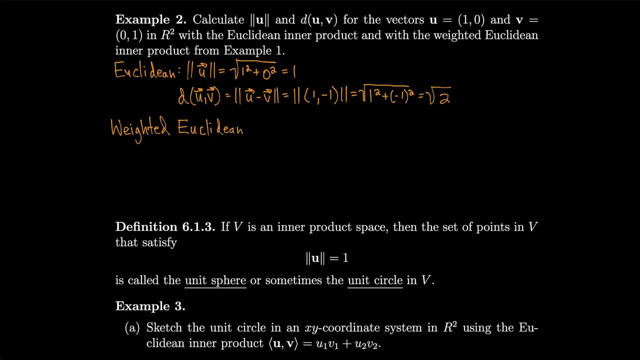 in the more general weighted Euclidean. It just shows a specific one. So we're looking at the length of u and that is going to be the weighted Euclidean interproduct of u with u, And I'll take the square root, Same thing as raising it to the 1 half power. 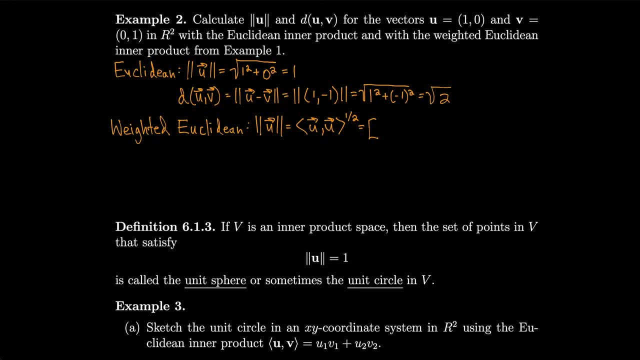 I'll just write it that way for some reason. So that's 3 times 1 times 1 plus 2 times 0 times 0 to the half power, which is 3 to the half power, aka the square root of 3.. 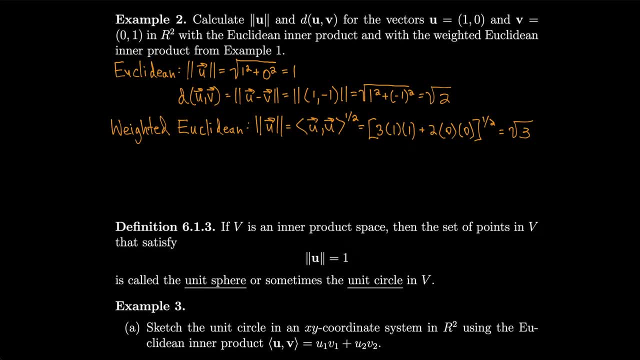 Okay, how about the distance? So the distance between u and v is equal to the length of u minus v, which is, let's see, the length. So take the interproduct of 1 minus 1 and 1. Raise that to the half power. 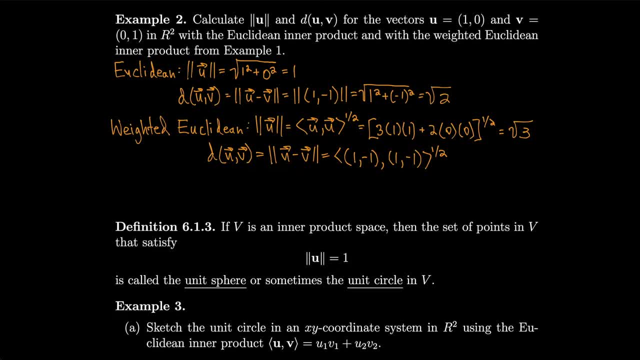 Write the same 1 minus 1 we were looking at before, But this time it's different interproducts. so it says that we should do 3 times 1 times 1 for the first component, plus 2 times minus 1 minus 1 for the second component. 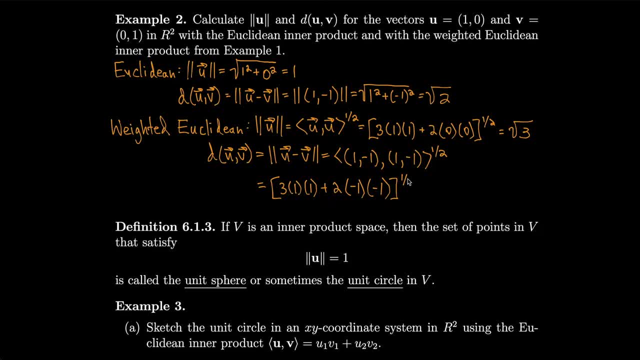 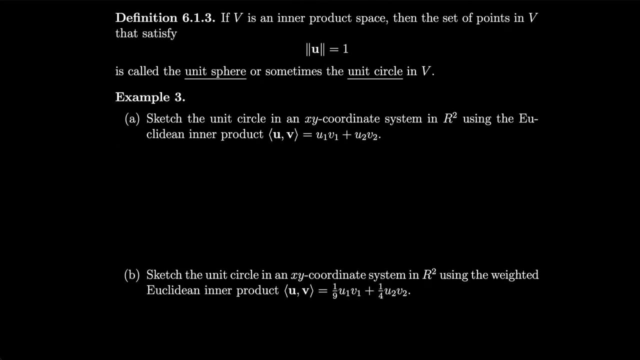 Raise that to the half power and we get the square root of 5.. So much different distance, much different length, depending on our interproduct chosen. If v is an interproduct space, then the set of points in v that satisfy the length of u equal 1. 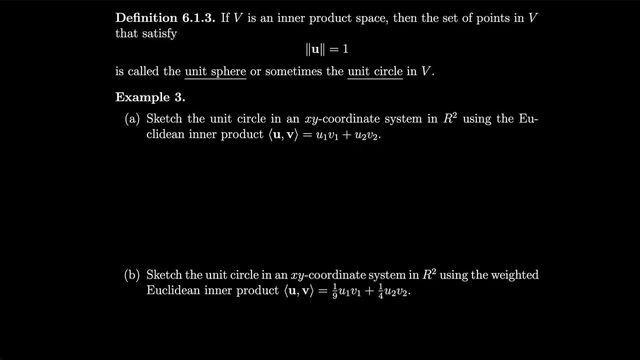 is called the unit sphere or sometimes the unit circle in v. So as an example, how about we sketch the unit circle in an xy-coordinate system in R2 using the Euclidean interproduct? So this is our standard unit. So we have, let's say, our vector. u is just equal to xy. 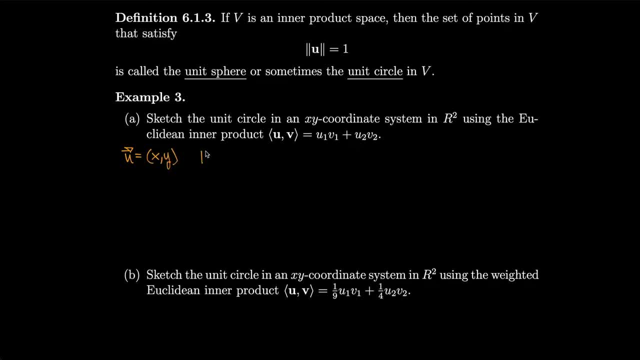 So we could look at it in the xy-plane. Then the length of u is equal to the Euclidean interproduct of u, with u raised to the 1 half. So that would just be the square root of x squared plus y squared. So if we have that equal to 1, then that's the same thing. 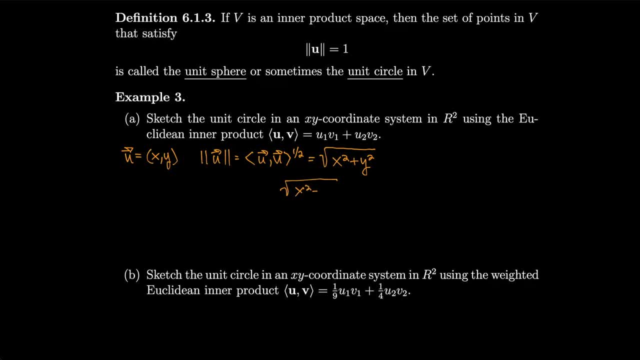 I'll just write it: the square root of x squared plus y squared equals 1 is equivalent to saying that x squared plus y squared is equal to 1, because it's just 1 squared if I square both sides. So hopefully you remember that is a circle. 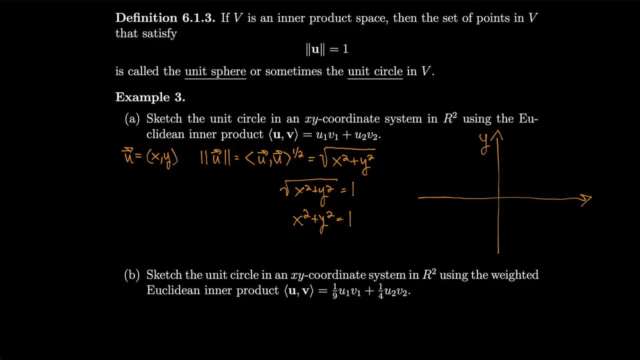 which is one of the reasons we call this the unit circle. So we have the vector u, length 1.. It points to all of these points that go around in a circle. Radius is 1.. Length of u is 1.. Okay, but how about if we use the weighted Euclidean interproduct? 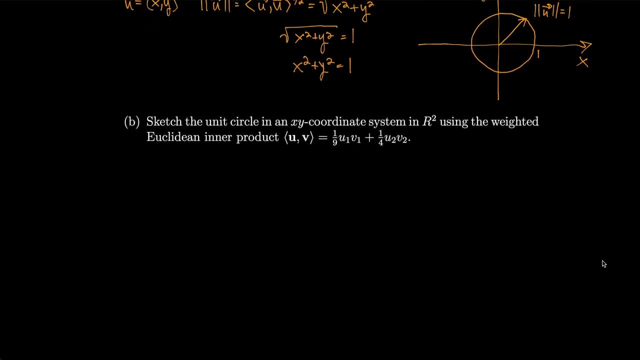 1 9th u1 v1 plus 1 4th u2 v2.. Well then, it'll look a little bit different. Let's set u equal to xy again And let's look at the length of u this time. 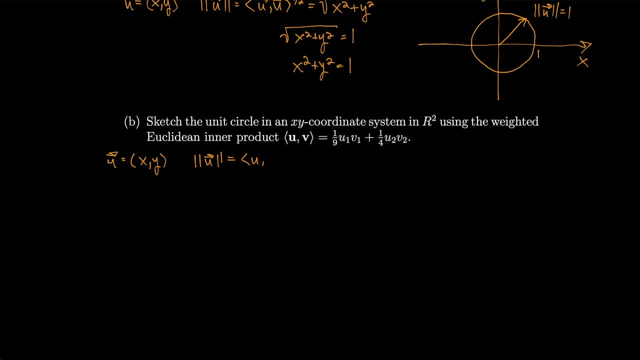 So remember, interproduct with a view with itself raised to the 1 half, And that's the same thing as the square root of u. So u1 is 1, 9th x times x is x squared. plus 1, 4th y times y is y squared. 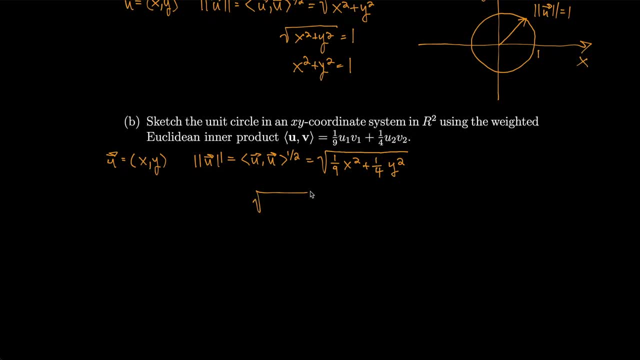 So a little bit different. In this case, if I set the square root of 1, 9th x squared plus 1, 4th y squared equal to 1, then I can square both sides and get x squared over nine plus x. 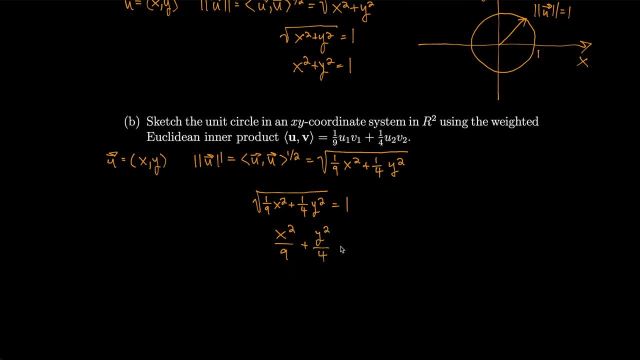 y squared over 4 equals 1, and our unit circle in the x-y plane ends up becoming an ellipse. So now we have. that's not so good. how about try a little bit harder? Not much better, but that's okay. Here's 3,, here's 2, right. 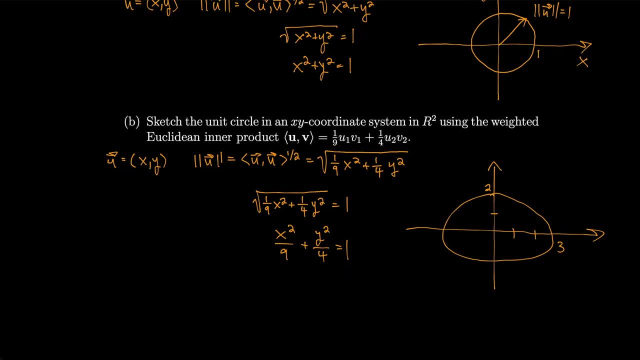 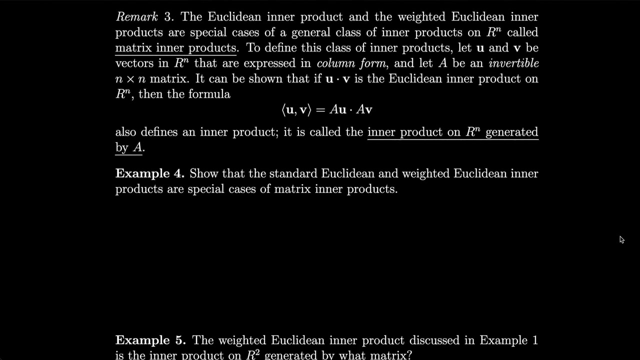 And here's an arbitrary vector with length 1 under this inner product. So the unit circle doesn't have to necessarily look like a conventional circle, depending on the inner product used. The Euclidean inner product and the weighted Euclidean inner product are special cases. 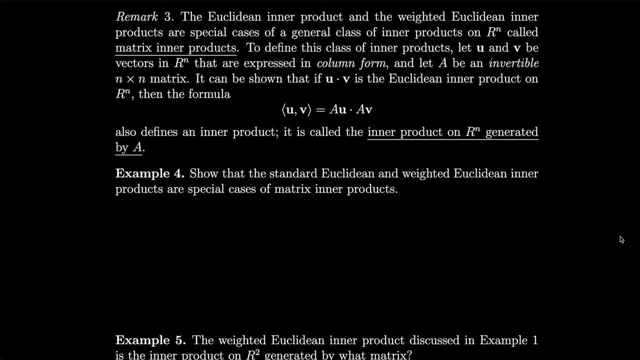 of a general class of inner products in Rn called matrix inner products. To define this class of inner products, let u and v be vectors in Rn that are expressed in column form and let a be an invertible n by n matrix. It can be shown that if u dot v. 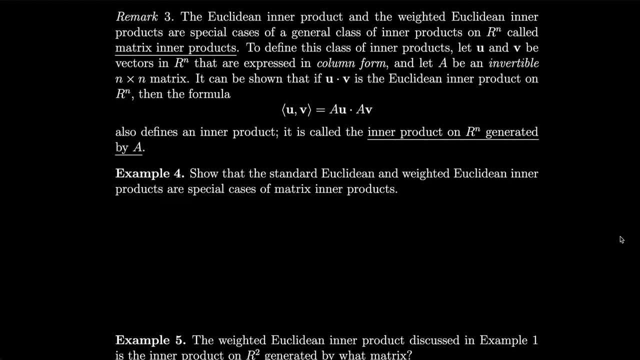 is the Euclidean inner product on Rn, then the formula uv equals au dot. av also defines an inner product. It is called the inner product in Rn generated by a. As an example, how about we show that the standard Euclidean and weighted Euclidean inner product 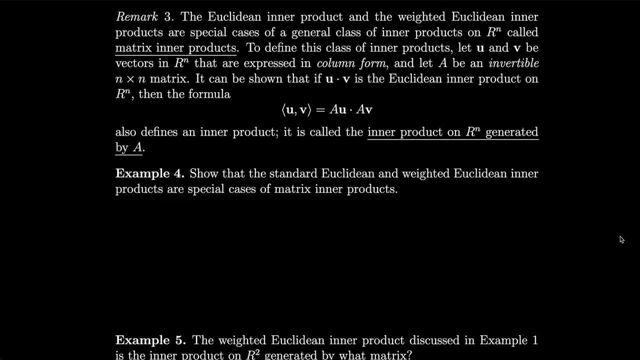 are special cases of matrix inner products. So let's look at the inner product of u and v. So that would be the identity i times, u dotted with the identity i dotted with v, which is u dot v, u dot v. in the case that we have the inner product generated by the identity. 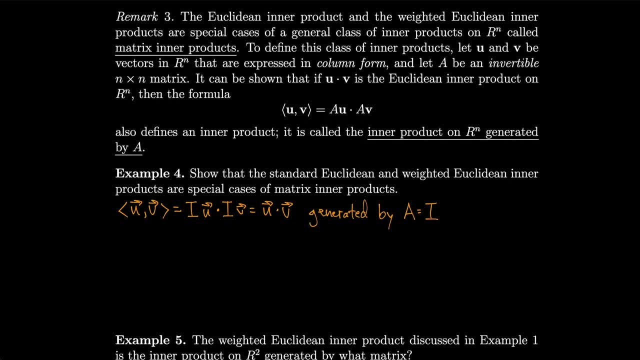 So we're setting a equal to i in this case. So if you set a equal to i in this equation over here, you just get the dot product. So that means the dot product is a special case of the matrix inner product with the identity chosen as the matrix. Let's see if we can get the weight of. 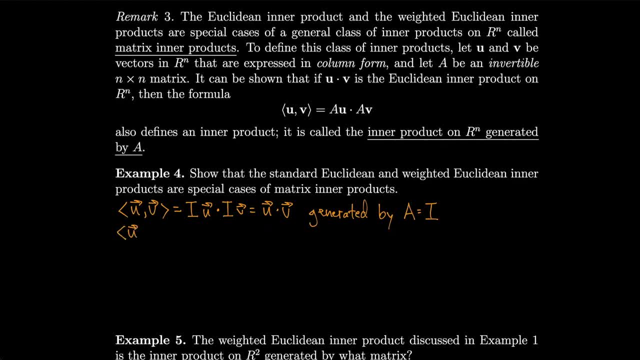 the Euclidean inner product. now, Well, the weight of the Euclidean inner product, that's w1,. oops, I need a w? w1, u1 times v1 plus w2 times u2 times v2, and so on. 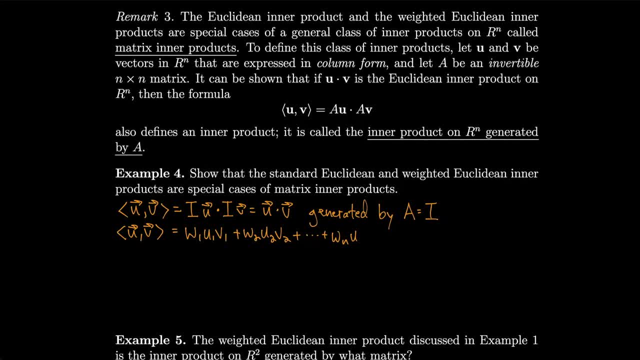 So we should end up with wn, un, n, vn. So that would be the inner product generated by the matrix A, where each diagonal entry is the square root of one of the w's, Because then if we take this matrix and multiply it through, the diagonal entries will end up with: 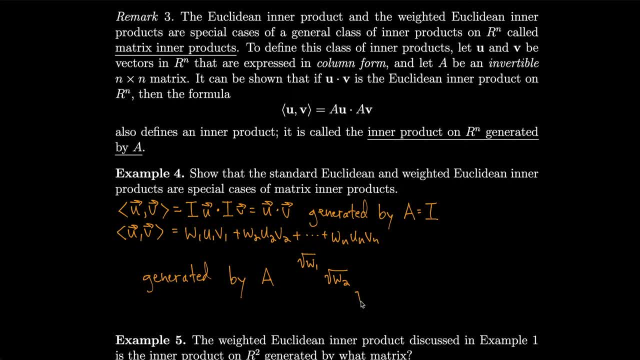 each successive component. So actually maybe I'll put zeros in the rest of it, so that way only the w's end up multiplying through. So we just get lots of zeros and I'll just keep going and placing w along the diagonals. 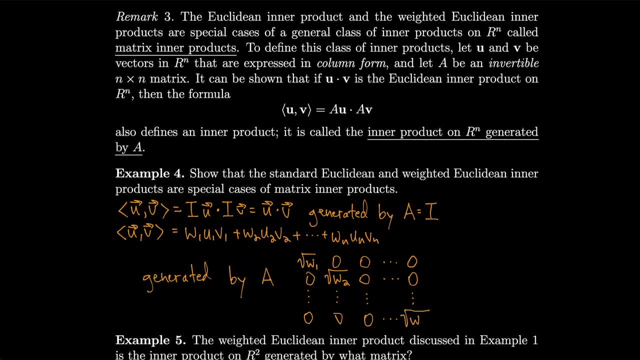 And I'll end up with the square root of wn. So if I took this matrix A and I multiplied it by u and I multiplied it by v and dotted them, then the square root of w1 multiplied by square root of w1 give me w1 times the first component. 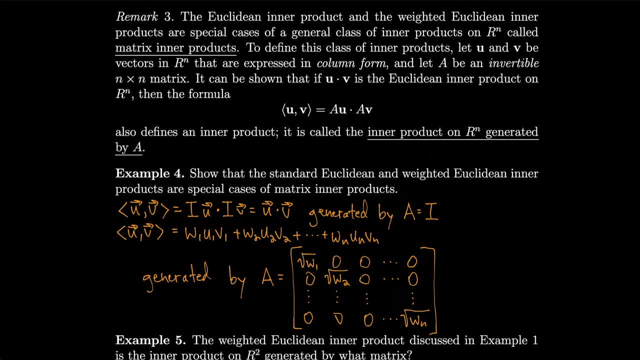 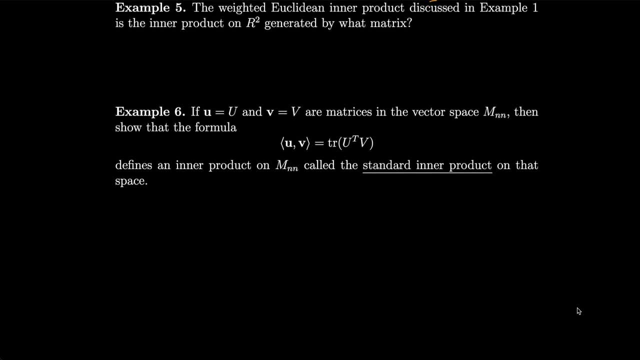 and so on. for each successive w along the diagonal, The weighted Euclidean inner product discussed in example 1 is the inner product in R2. generated by what matrix? Well, let's write it out. We had uv equal to 3u1 v1 plus 2u2 v2.. So that is generated. 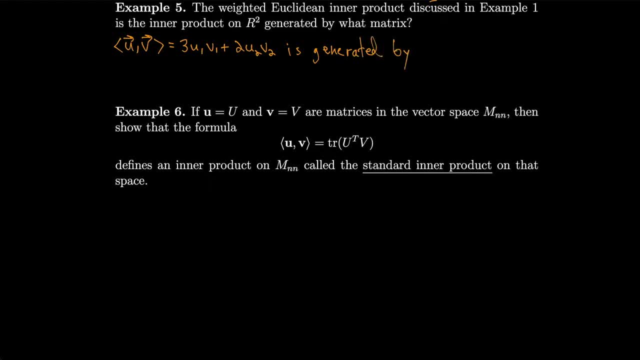 by the matrix A, equal to the square root of the w's and diagonals right. So the first w is 3, so I'll take square root of 3.. The second w is 2.. Let's take square root of 2, put those diagonals, put zeros elsewhere, and that's how we can. 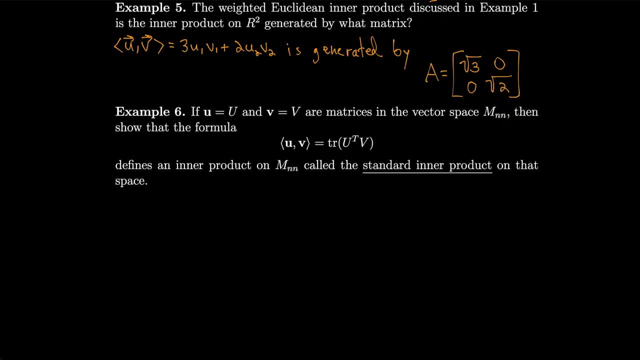 build our matrix A. If u equals u and v equals v are matrices in a vector space, MNN. then show that the formula uv equals the trace of u transpose times. v defines an inner product of MNN called the standard inner product on that space. Okay, let's set u equal to an arbitrary matrix. How about we do it two by two? 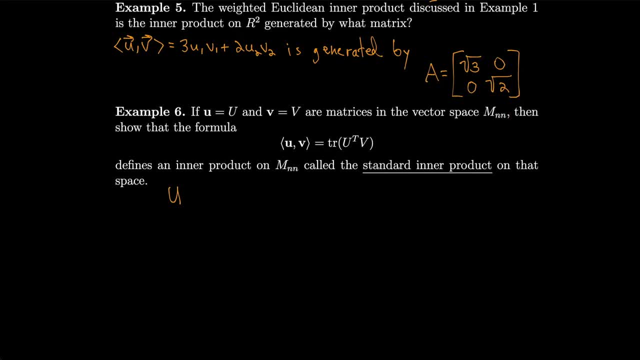 and we'll pretend that we did it for n by n, because it could generalize fairly easily. So I'll have u1, u2, u3, and u4 as the components of, as the entries of this matrix, And I'll have v equal to the matrix v1, v2, v3, v4.. 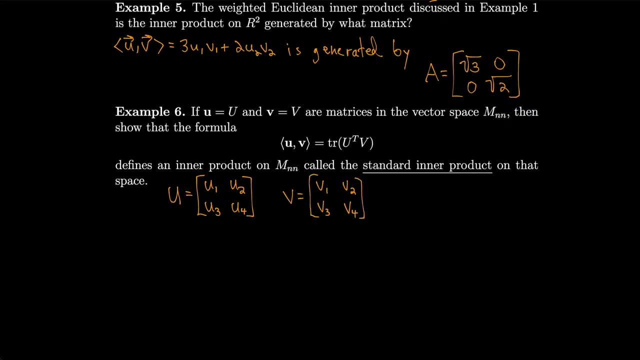 Let's look at the inner product of u with v. So in this case that's the trace of u transpose v. Okay, so if we take u transpose so it switches these guys right, because this first row becomes the first columns. the u moves out over here the u2, but u1 stays over here where we do the trace and u4 stays in the middle where we do the. 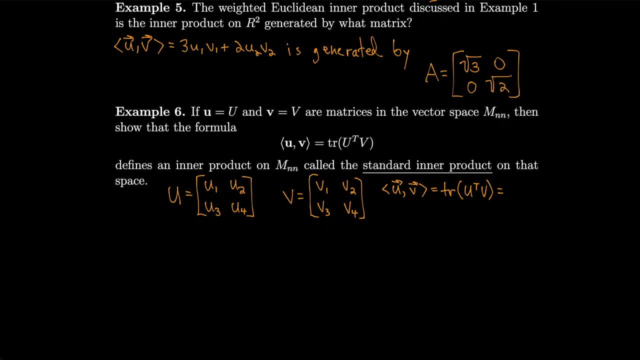 But u2,. u1 stays over here where we do the trace, and u4 stays in the middle where we do the trace, the dash, and u4 stays to my upper over here when we do the trace, so the diagonal entries don't change. Remember, though, that when 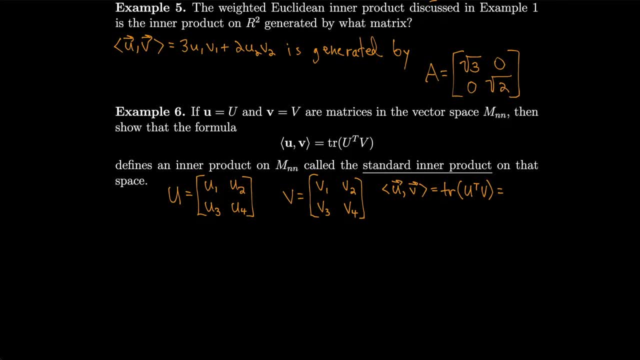 we multiply matrices, we do it row and by column. We do the row in one matrix times the column in the other. So if we're interchanging rows and columns in one of the matrices and the diagonal numbers don't change, then the u1 will multiply by the v1, but then u3 will end up over here at u2. 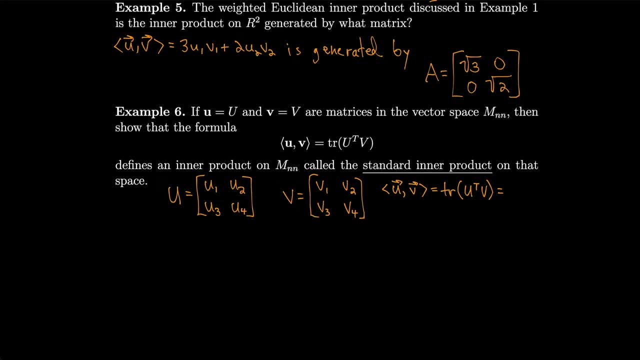 so it'll multiply by v3, because it'll be in the first row. so it'll multiply by the first column. So we'll have u1 times v1 plus u3 times v3 for the first entry in the product and similarly for the other diagonal entry that we need in order to do the trace. 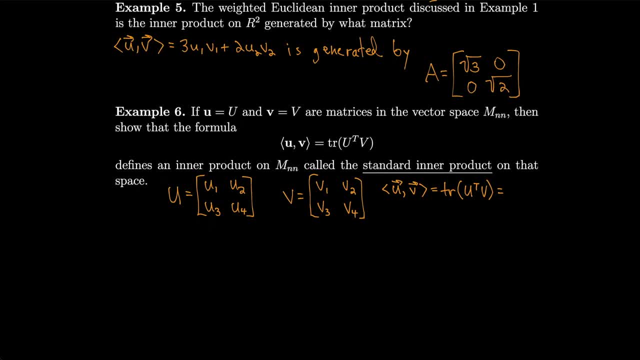 we'll end up with u2 times v2 plus u4 times v4.. So that's kind of cool and it makes a little more sense now why we chose this strange formula to be the standard inner product on the matrix vector space mnn. So we'll get u1 v1 plus u2 v2 plus u3 v3. 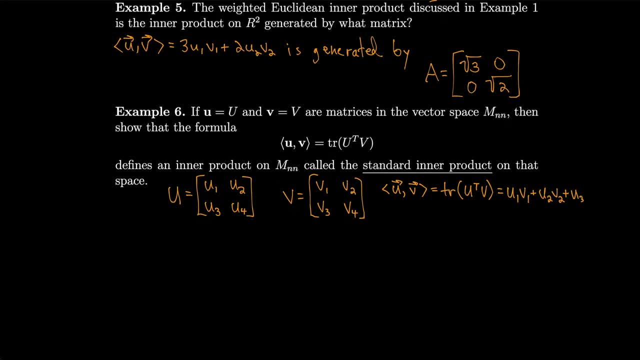 I don't like that. u plus u4, v4 and we'll look at the length of u, so that would be the square root of the inner product of u with u. so that's the square root of the trace of u. transpose times u, so that's the square root of u1 squared plus u2 squared plus u3 squared plus u4 squared. 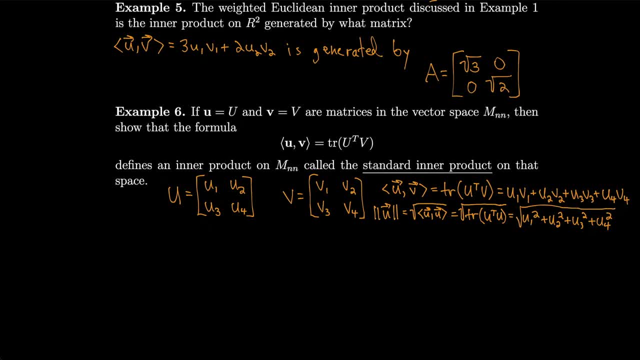 okay, let's set u and v into some. okay, let's set u and v into some specific matrices. just as an example, how about I take u equal to the matrix, u equal to say 1, 2, 3, 4. make it a little more concrete, I'll take v equal to the. 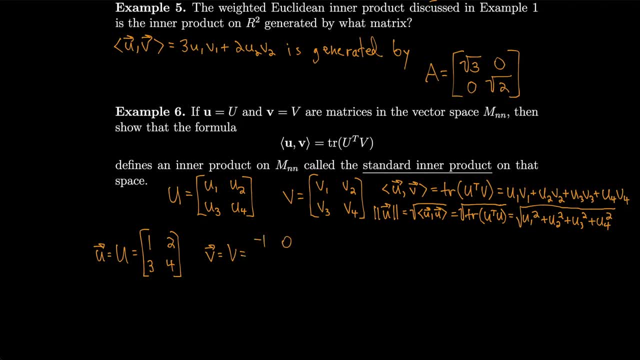 matrix v equal to minus 1, 0, 3, 2. then if I look at the inner product, then that's just the trace: of u transpose v, so that's one times minus 1 plus two times zero, plus three times. oh, and also now I get the line. 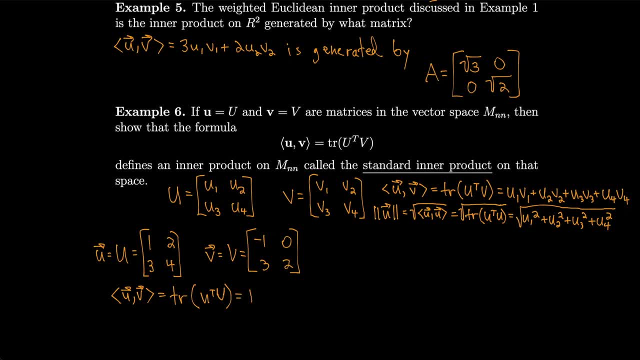 Okay, I always think of these entrepreneurs as against each other and I do those very long oaths, of course. four times 3 plus 4 times 2.. So you can see that the reason why we use this formula is just to get all of the corresponding components multiplied together. If I want. 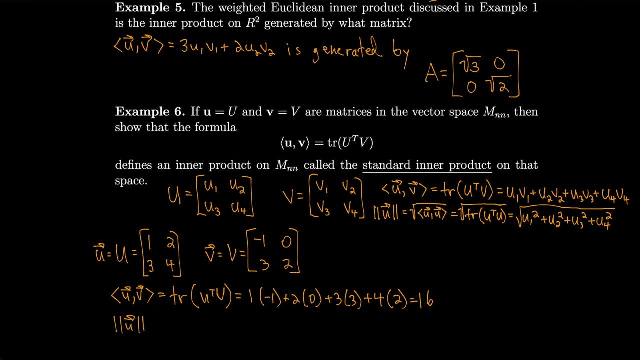 the length of u, then that would just be the square root of the inner product of u with u. So that's the square root of the trace of u. transpose u, which is the square root of 1 squared plus 2 squared, plus 3 squared plus 4 squared, So that's. 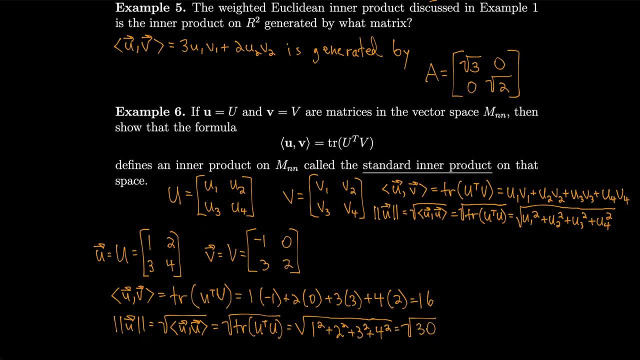 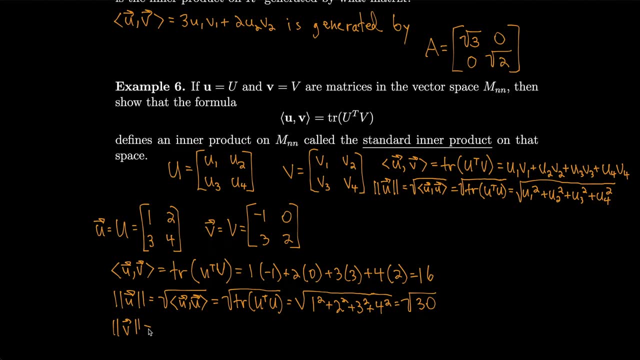 square root of 30.. If I wanted the length of v, I could similarly get it Square root of inner product of v with v. So that's the trace of v. transpose times v, which is the square root of minus 1 squared plus 0 squared. 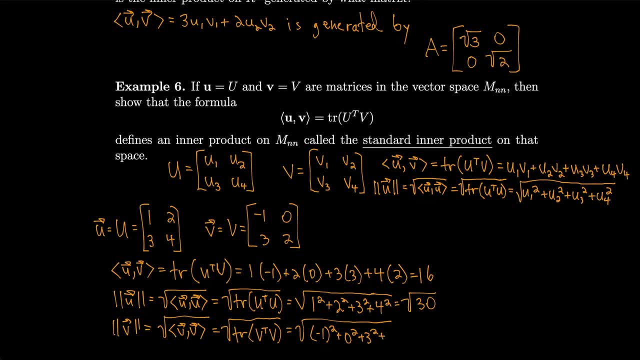 plus 3 squared plus 2 squared, which is the square root of 14.. So to really correctly answer this example, we would, in order to show that the formula defines an inner product on 99N, we would have to go through each of the inner product axioms. I'm not going to do that because I think that, given this, 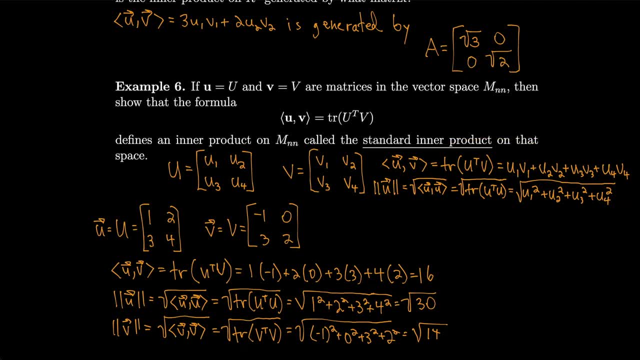 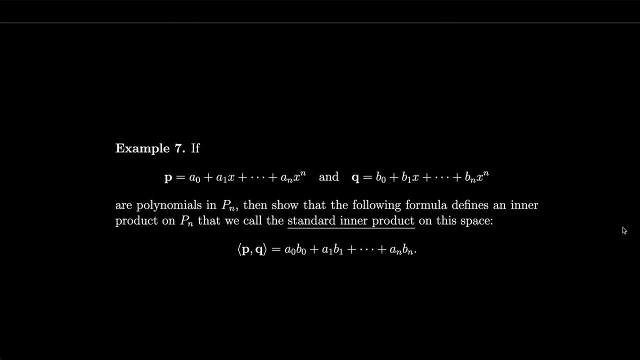 example, and given this explicit formula for the inner product, you can see that it's basically just a dime dot product on the components And, as we saw previously, the dot product is definitely an inner product. Oh, and also clearly it generalizes to NN. 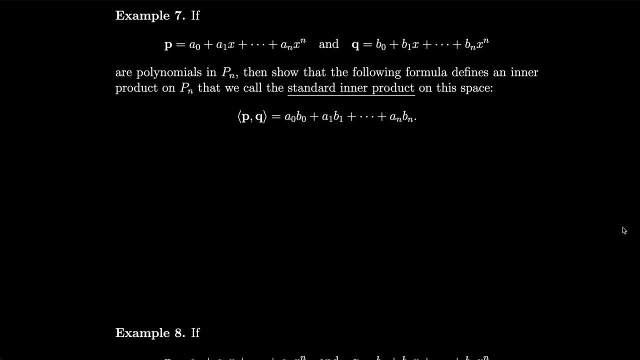 you know, for the same reasoning as in the two by two case. Let's move on to this next example. If P and Q are polynomials in PN, then let's show that the following formula defines an inner product in PN that we call: 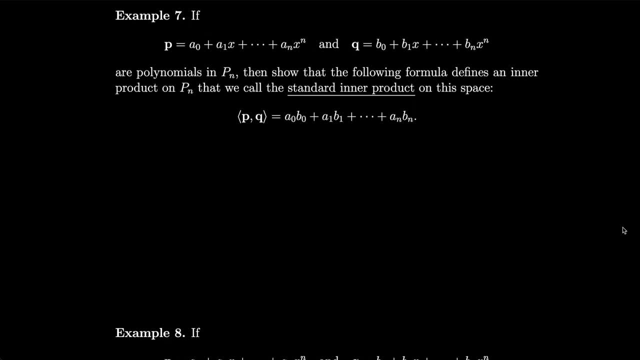 the standard inner product on this base. So we take each of the coefficients and we multiply them and then we add them up. So all of these are pretty similar to the dot product that we're used to, Just we have to adjust it slightly. 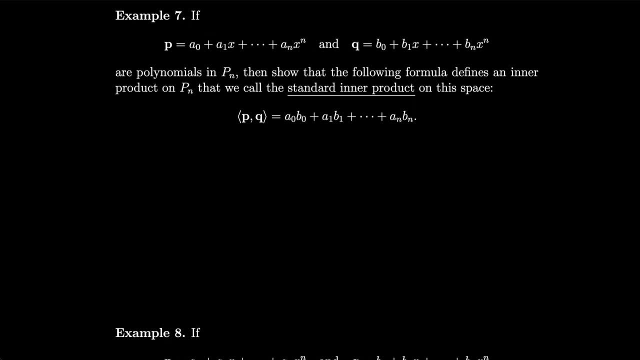 you know, so that it ends up looking like a dot product in the end. By the way, look at the length. The length of a polynomial under this inner product would be equal to the square root of each of the coefficients squared, So that would be A0 squared plus A1 squared. 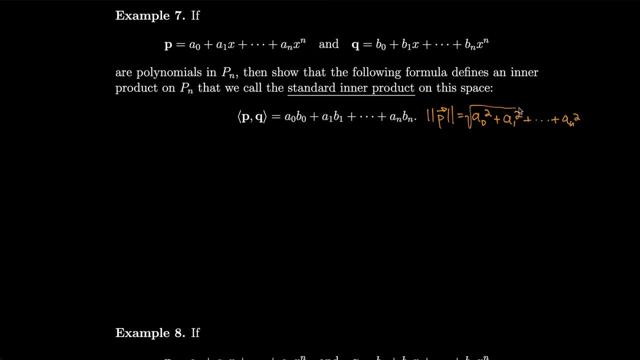 and so on through AN squared. OK, let's check each axiom for this example. So let's do number one. We're looking at P, the inner product of P, with Q, So that's equal to A0, B0, plus A1, B1, and so on through AN BN. 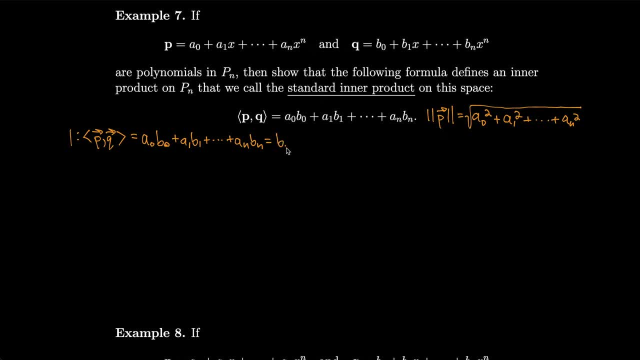 And that's equal to the same thing if we switch it B0, A0, because multiplication for real numbers is commutative. So B0, A0 plus B1.. B1, A1, and so on. We just swap A's and B's, which gives us 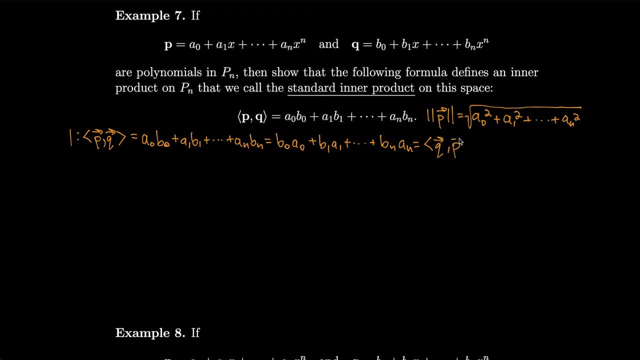 the inner product of Q with P. So first axiom is good, Let's do the second. Let's set some R equal to C0 plus C1x plus C1x. So we're going to do the same thing. So let's do the same thing. 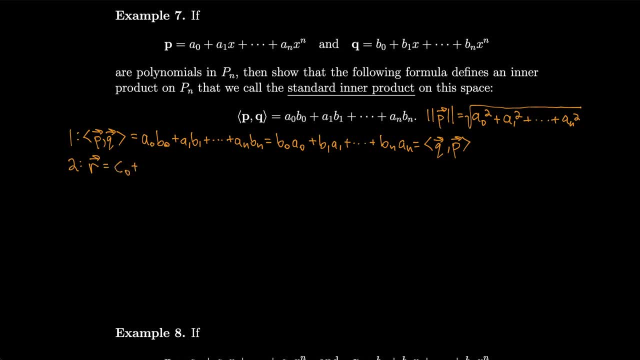 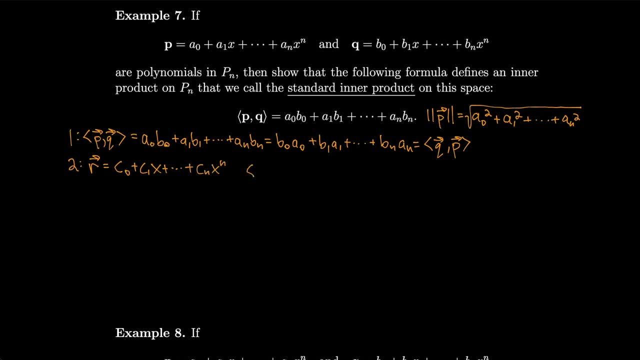 and then I'm going to work out one derivative, And so that will make that solution simple enough to be able to do this pretty easily. So let's do this, Because do perm unquote charge. So let's just do this, OK. 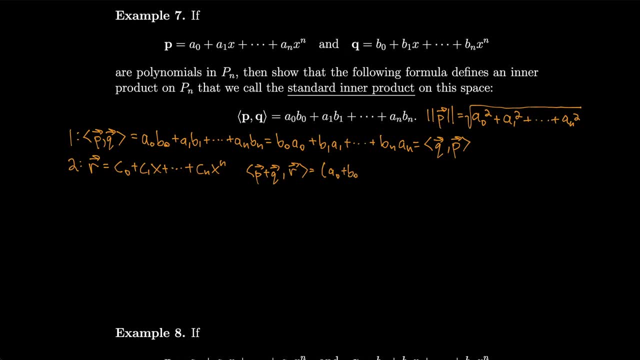 I'm going to use P and P1.. Let's do this And I'm going to be able to do this. So let's put it down into the common formula from the everywhere combination of p to R, And I'm going to do a new polynomial of P and Q. 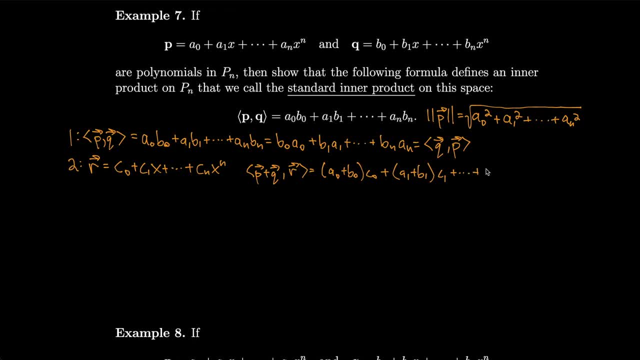 And that will make this expressions. So on until we get to an plus bn times cn, We'll set that We'll distribute the c's. It's pretty similar to what we did before when we were proving this axiom. So we're proving the axiom holds in the other case that we did. 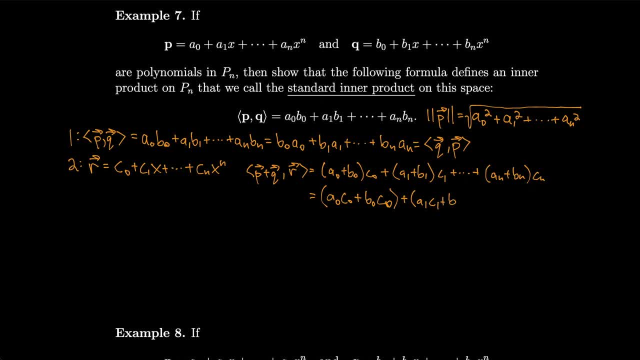 So we distribute it, We get a1 c1 plus b1 c1,, all the way through an cn plus bn cn, And that'll equal a0 c0 plus a1 c1, and so on an cn. So plus b0 c0 plus b1 c1,, all the way through bn cn. 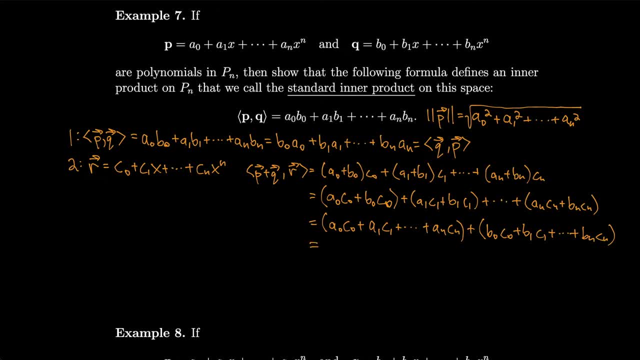 And I separate it that way so that I can view it as two new inner products. We have now the axiom holds. We have the inner product of p with r and the inner product of q with r. OK, Let's check the third axiom now. 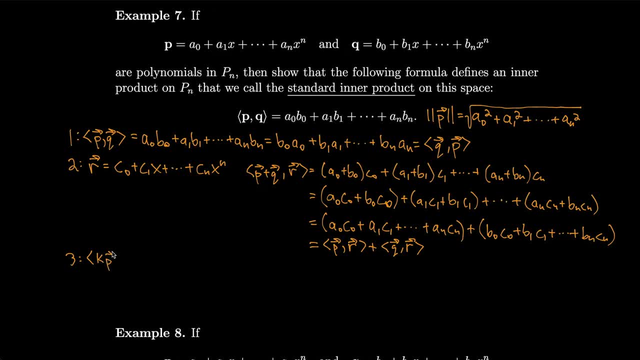 So we're looking at some constant k times p, inner product with q, So that's k, And then we get k times a1, b0, plus k times a1, b1, and so on all the way through. k times a1, b1, I'll factor out k. 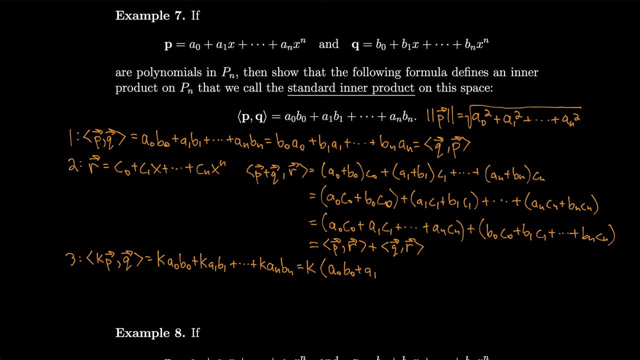 I'll get k times a0, b0, and so on, All the way to k times an- bn. I'll factor out k. I'll get k times a0- b0. Plus a1- b1.. All the way through a1- b1.. 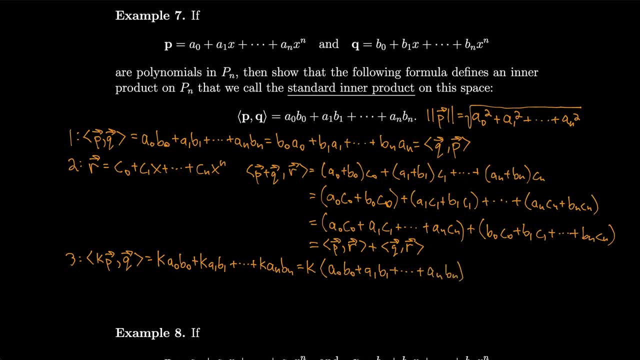 way through a and bn, which is just k times the inner product of p with q. OK, number four, Let's check the inner product of p with itself. So that's a0 squared plus a1 squared, all the way through an squared. 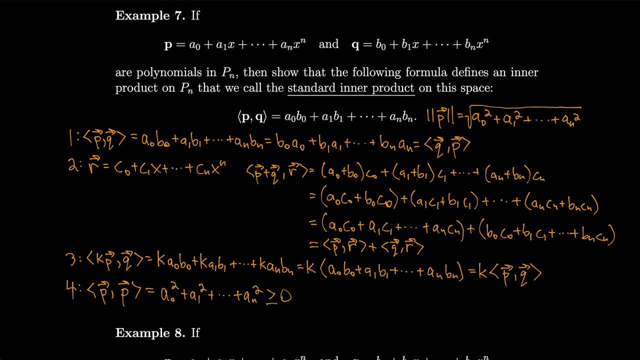 And all those are squares, so they have to be positive or greater than or equal to 0, not negative. Let's look at the inner product of p with itself. That has to be 0 if, and only if, all of those coefficients are 0.. 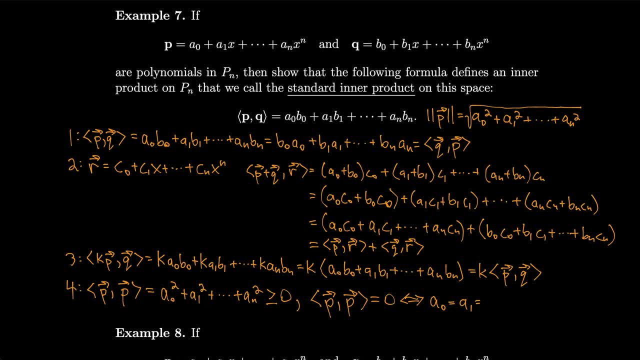 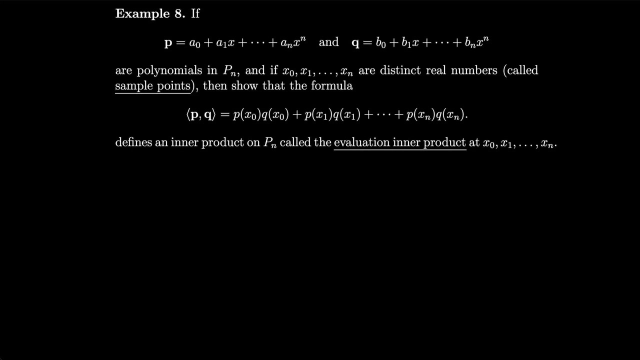 So a0 has to be 0,, a1 has to be 0, and so on, which is the same thing as saying that p would have to be 0. The entire polynomial would have to be the 0 polynomial Next up if p and q are polynomials in pn. 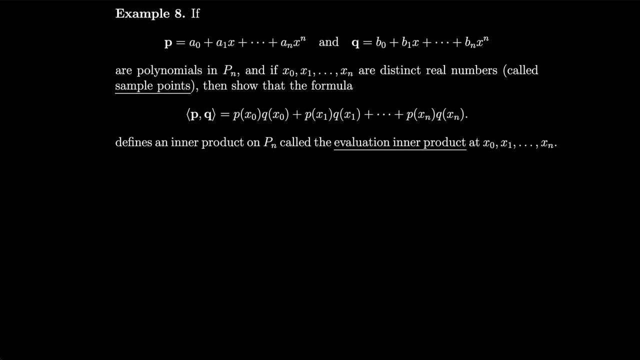 and if x0 through xn are distinct real numbers, called sample points, how about we show that the formula pq equal to p evaluated at x0, q evaluated at x0, plus p evaluated at x1 times q evaluated at x1, and so on? 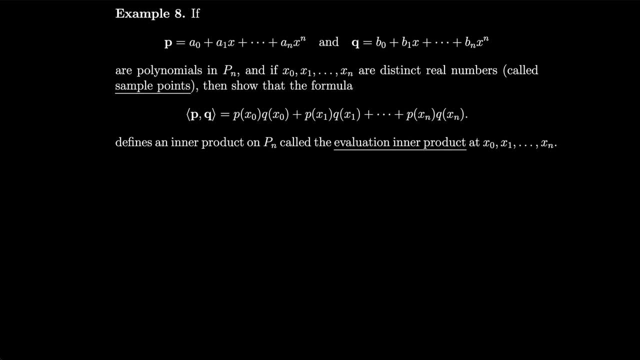 defines an inner product on pn, called the evaluation inner product, at x0 through xn. Well, first of all, 1 through 3. Follow immediately from properties of the dot product similar to the matrix example that we looked at. When you evaluate polynomials at numbers, 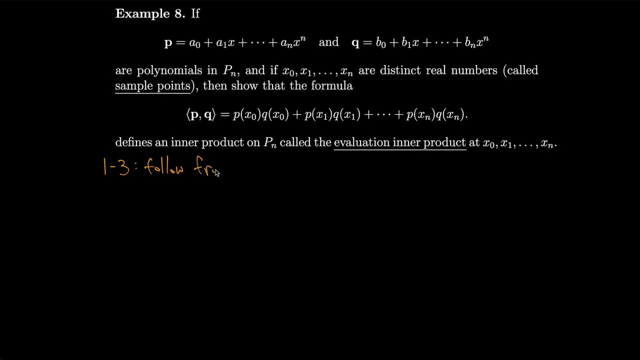 they just become numbers. So 1 through 3 are pretty clear. There really is only one spot here we have to be careful, and that's with property number 4, because with property number 4, we have that we have to have the inner product equal. 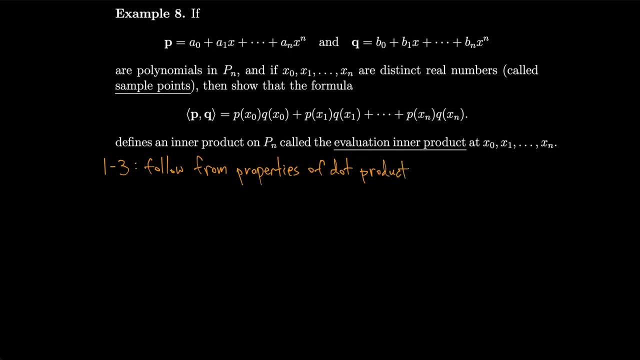 to 0, if, and only if, the polynomial is 0. So we just have to verify that. So let's go through 4 carefully. First, if we take a polynomial and we look at the inner product of that polynomial in itself under this evaluation- inner product. 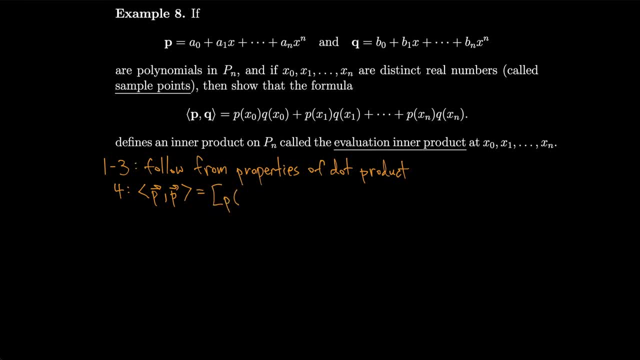 then that's just the same thing as taking the polynomial evaluated at x0. And squaring it. Squaring that, adding it to the polynomial evaluated at x1, squaring that and so on all the way through xn And all those squares will clearly 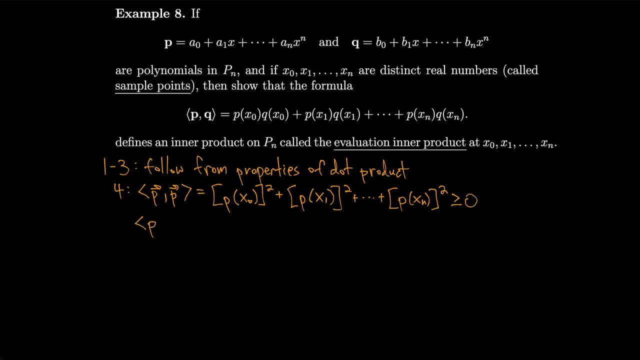 have to be greater than or equal to 0,, as we've already seen. So let's look at the interesting case where we have the inner product of a polynomial to polynomial equal to 0.. So that means that the polynomial evaluated at x0. 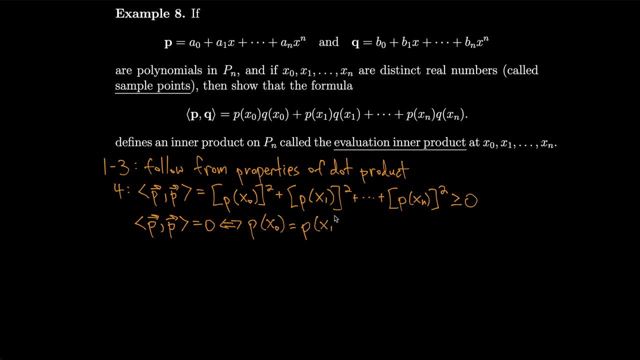 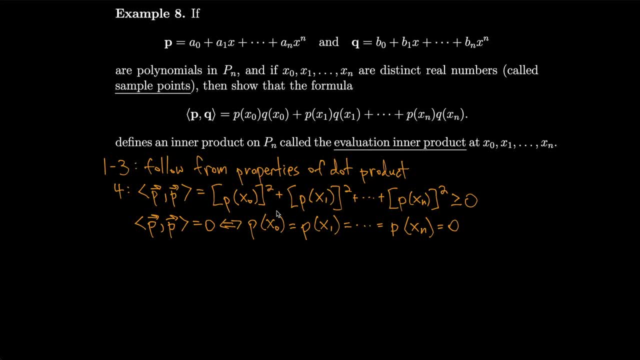 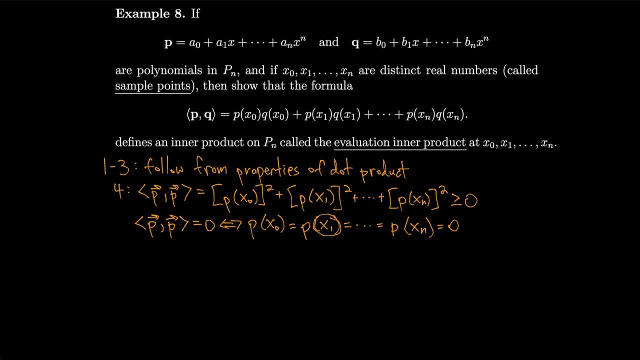 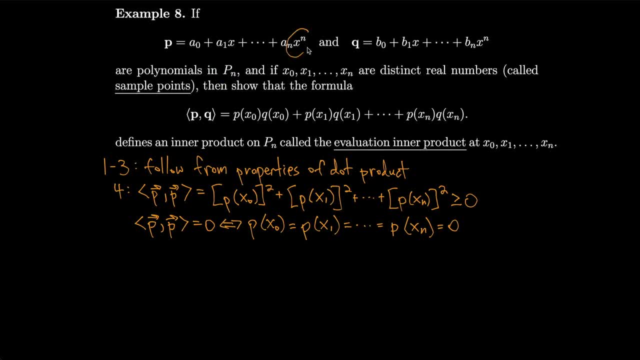 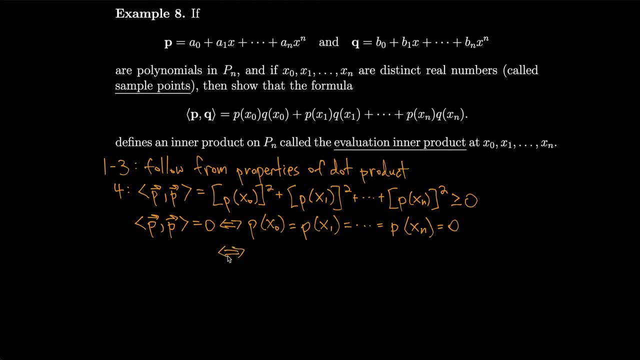 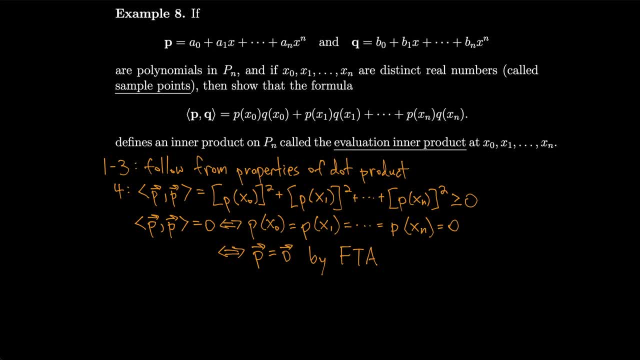 So, So, So, So. OK, so now we've shown that the evaluation product is actually an inner product. Notice that the length of a polynomial p under this inner product is just equal to the square root of the inner product of the polynomial with itself. 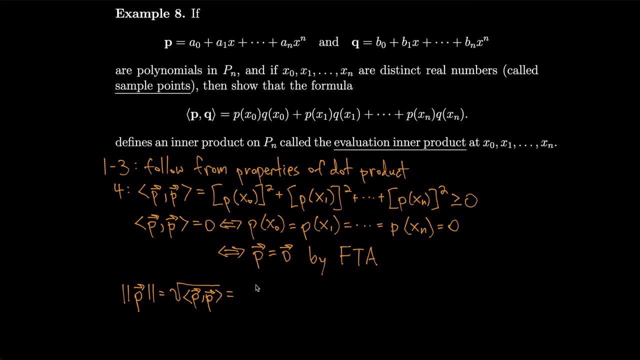 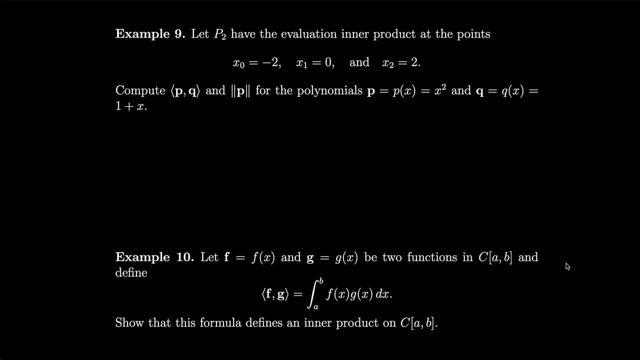 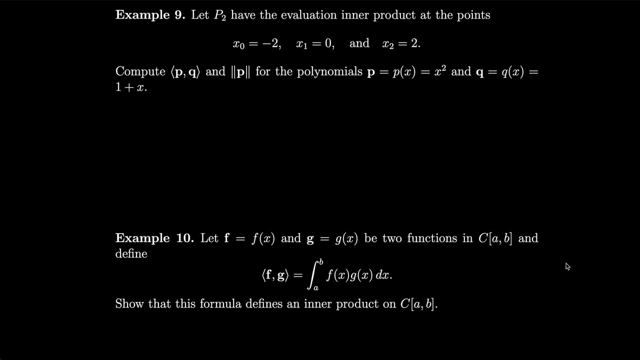 So that means that it's equal to the square root of p evaluated at x zero squared, plus p evaluated at x1 squared, and so on all the way through p evaluated at xn squared. How about we let p2 have the evaluation in a product at the points x0,, x1, and x2 given? 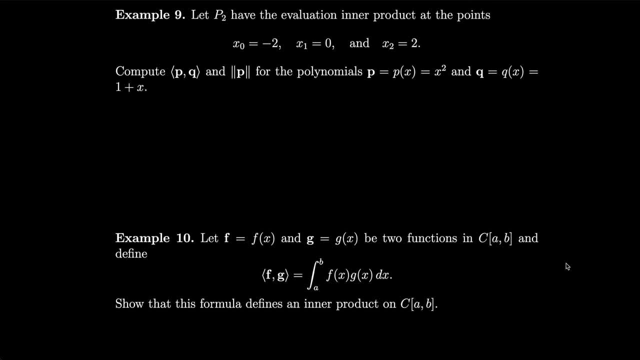 and let's compute pq and the length of p for the polynomials p and q given. So what we'll do is we'll write out pq so that's equal to p evaluated at. let's see, the points are minus 2,, 0, and 2.. 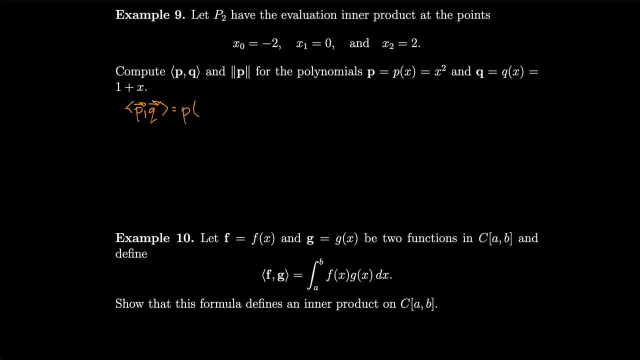 p is x squared. so that means what we'll do is p of minus 2 times q of minus 2 plus p at 0 times q at 0, plus p at 2 times q at 2.. Okay, so p at minus 2 is x squared at minus 2, so negative 2 squared is 4,. 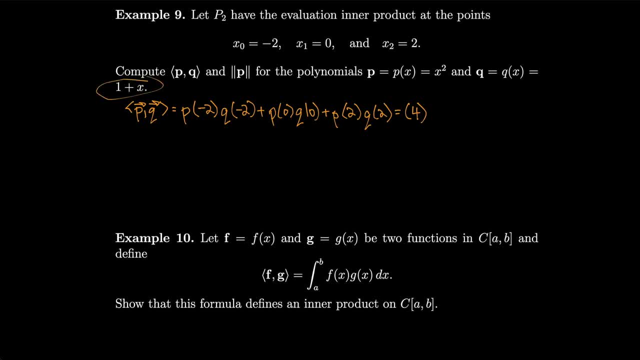 and then q is 1 plus x, So 1 plus negative 2 is 1, minus 2 is minus 1, plus p at 0, 0 squared is 0, and then 1 plus 0 is just 1 for q, and then 2 squared is 4, and 1 plus 2 is 3.. 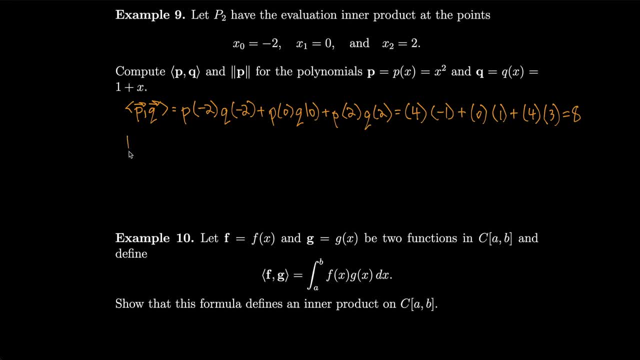 Adding all that up we get 8.. Now let's get the length of p. So we'll take the square root of p at x0 squared, plus p at x1 squared, plus p at x2 squared, And our first point was minus 2, so that's p of minus 2 squared plus p at 0 squared, plus p at 2 squared. 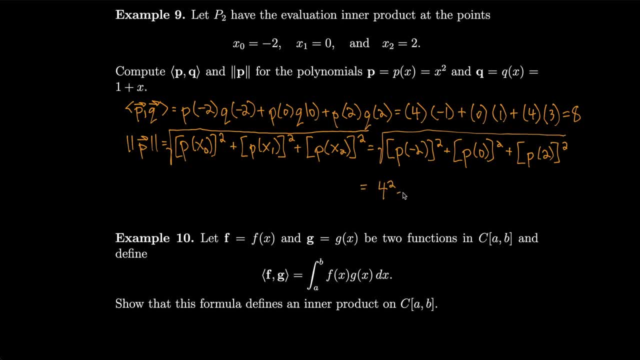 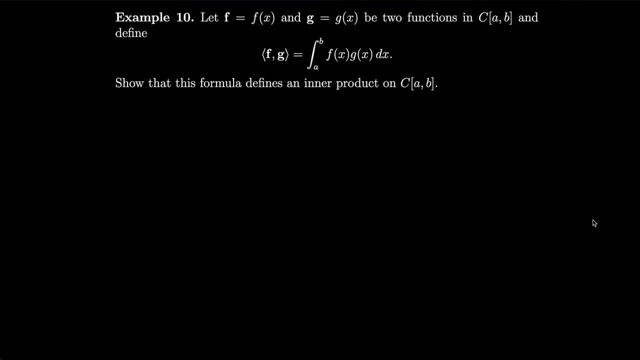 So we get square root of 4 squared plus 0 squared plus 4 squared, So that's the square root of 32, which is 4 radical 2. How about we let f and g be two functions that are continuous in the interval a b? 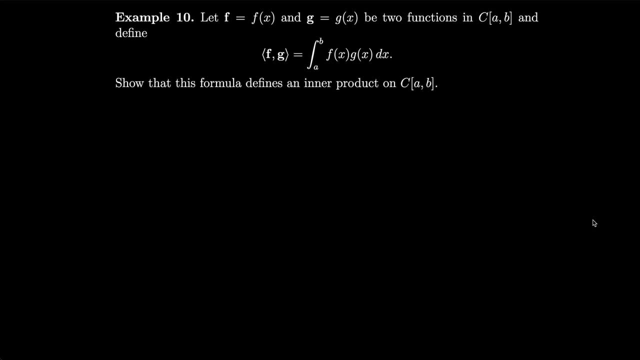 so they're in c a, b and let's define that inner product as the integral of the product Of the two functions, And we'll show that this formula actually does define an inner product on c a, b. So let's look at each axiom. 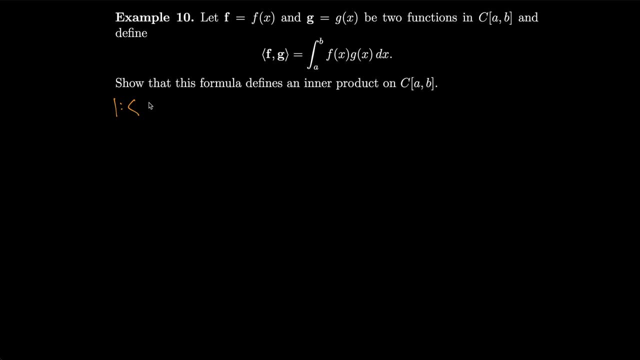 For number 1, let's look at the inner product of f and g, So that'll be equal to the integral from a to b of f of x times g of x dx. But Multiplication of functions is commutative, So that's the same thing as the integral from a to b of g of x times f of x dx. 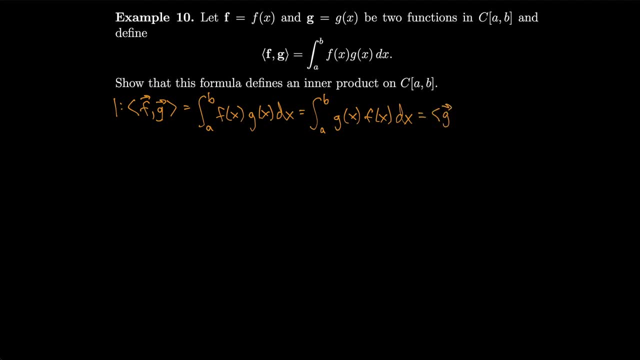 So that's just the inner product of g with f. So the first axiom is done. That was easy. Let's look at the second one. Let's look at f plus g And we'll take that inner product with another function. Let's say h. 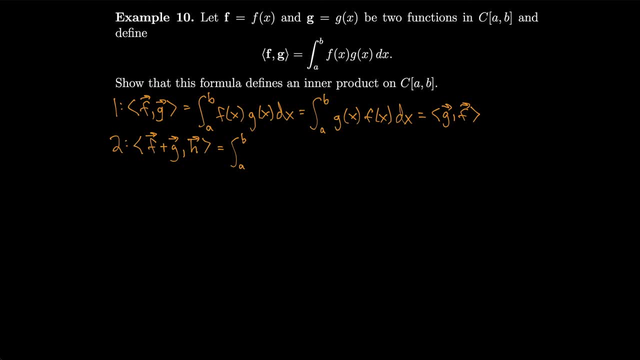 So that would be the integral from a to b Of f of x Plus g of x Times h of x dx, And that's equal to the integral from a to b of f of x times h of x, h of x dx, plus the integral from a to b of g of x times h of x dx. 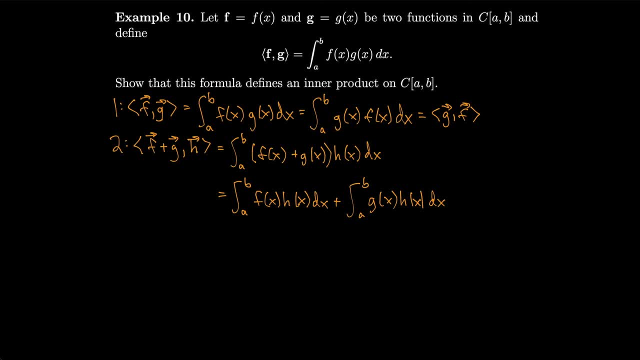 because all we did was distribute h and then apply the linearity property of integrals to separate out the two integrals. so that's just f, h, the inner product, and add it to the inner product of g with h. okay, let's look at number three. 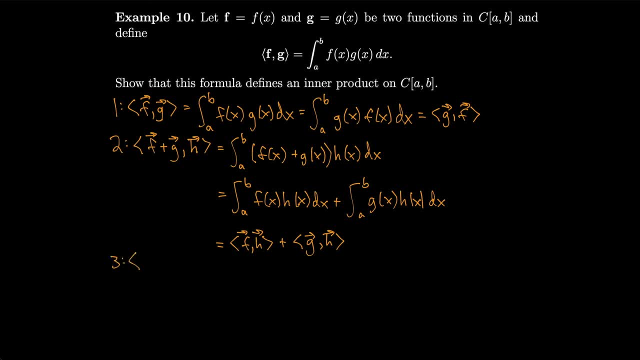 if we take a constant times f, we take that inner product with g. that's the same thing as the integral from a to b of k, f, of x, g, of x, dx, and again by linearity we could pull out the constant, so that's k times the integral of f, of x, g, of x, dx. 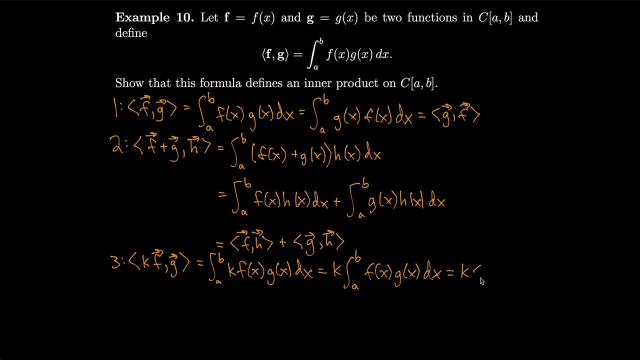 which is just k times that inner product. so that takes care of number three. lastly, number four: if i look at the inner product of f with f, then that's the integral from a to b of f, x times f of x, or f squared x dx. 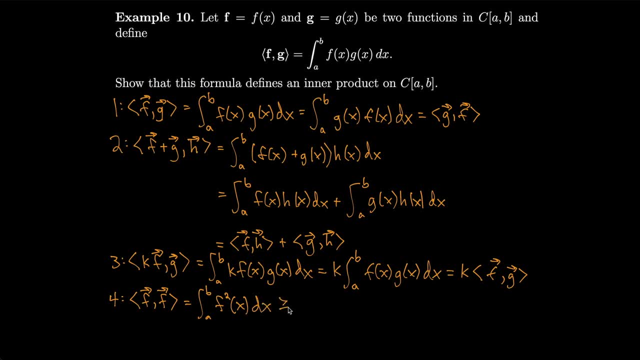 if you like that notation which has to be greater than or equal to zero. anything times itself. any square is going to be greater than or equal to zero to 0, and then the integral of that would have to be greater than or equal to 0.. 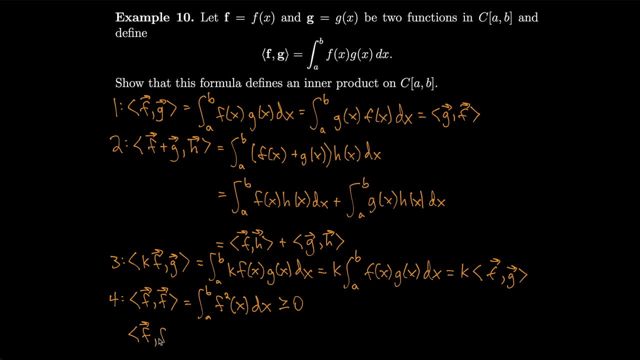 How about the? so that means that the inner product of f with f can only be equal to 0 if, and only if, because, remember, the integral can only be 0 if the function is 0 on the interval. So that was a, b, but that is only the case. 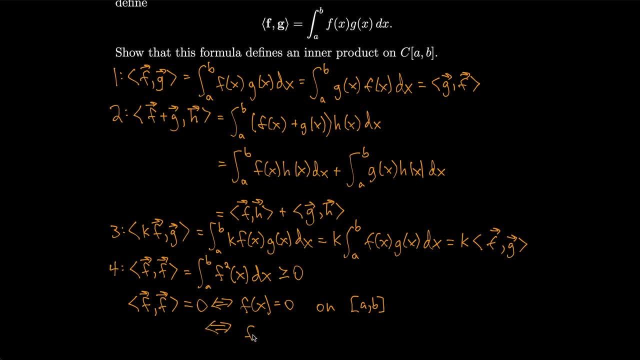 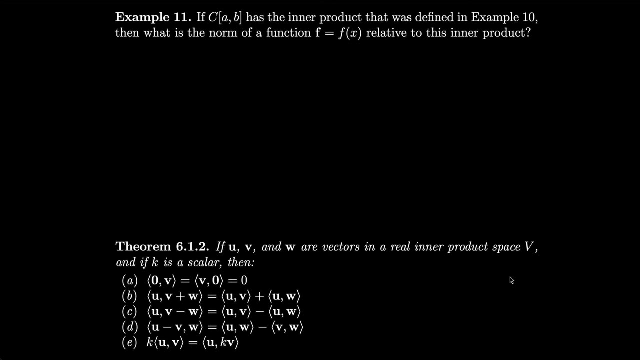 if, and only if, we have f equal to the 0 vector. If f is a 0 function, f is a 0 vector. If c, a, b has the inner product that was defined in example 10,, what is the norm of the function? 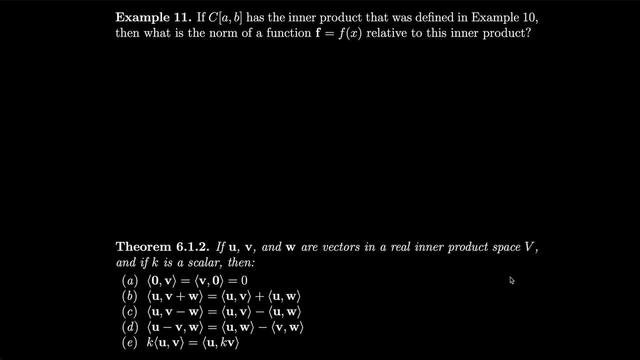 f relative to this inner product. Well, let's see, The norm of f is equal to the inner product of f, with itself raised to the half power, which is just, by definition of the inner product that we're given, equal to the square root of the integral from a to b. 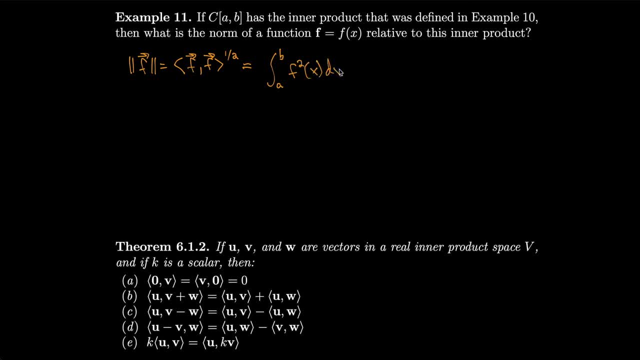 of f squared of x, dx. Well, that's kind of cool, but that means that, even though they didn't ask, but the unit sphere in this case would be equal to the set of all of the functions f that are inside of c, a, b. 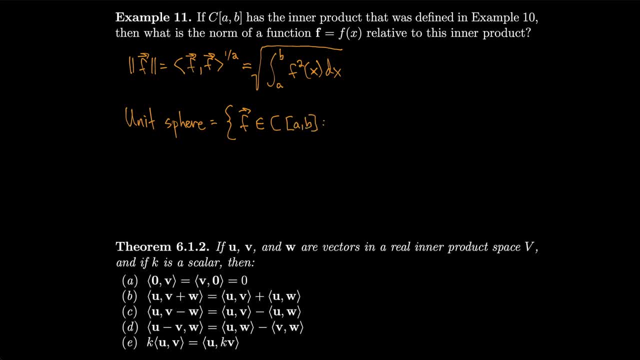 So all of the functions continue with this kind of inflexible integral. So that is one way you can calculate the length of the integrals throughout, the effect of the integral. So if you look at this on a, b, such that when you take their integral, 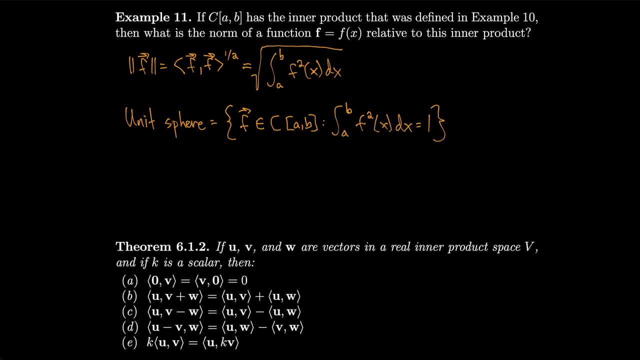 of the f of x square dx, you get one. So not exactly what you would expect from the unit sphere, unit circle. it's an interesting inner product because in calculus- and I'll write as an aside that this is not equal to the length from calculus- 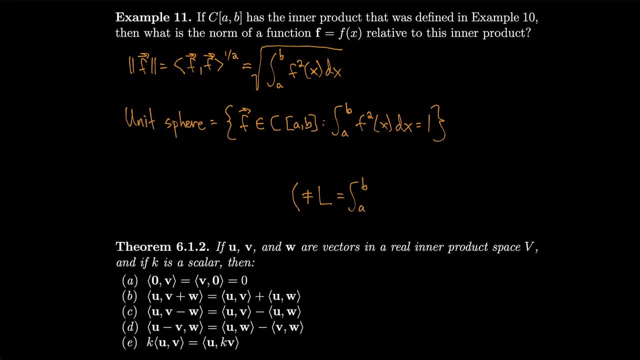 which is defined as the integral, from a to b, of the square root of 1 plus the derivative squared. So we have to be a little bit careful here, because in this case the vector length that we look at in relative magnitude, relative to our inner product, is very different than the. 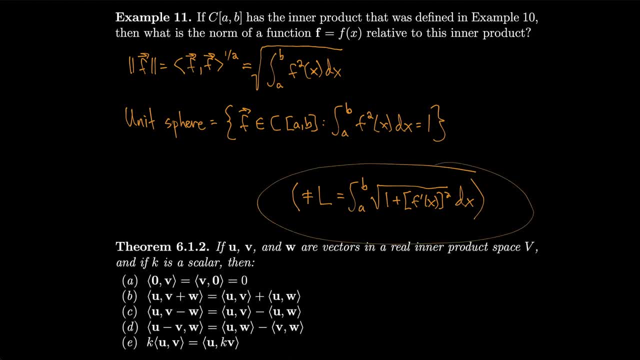 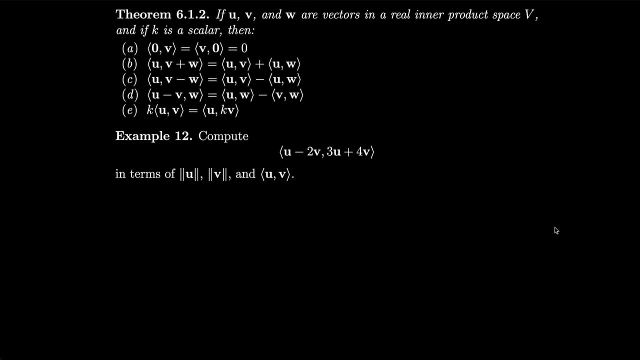 length that we're kind of used to from calculus, which is the arc length given by the integral of the square root of 1 plus the derivative squared. This is the function squared. this was the derivative squared. If u, v and w are vectors in a real inner product space, v. 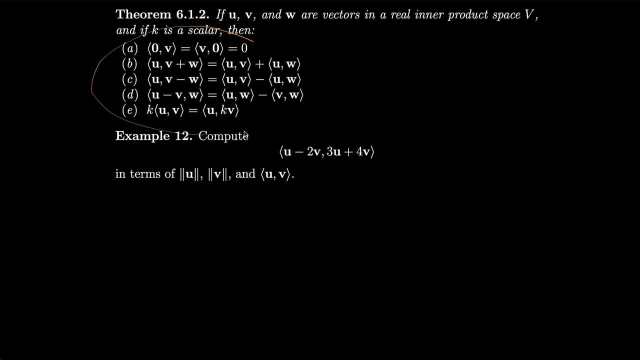 and if k is a scalar, then we have all these properties over here and we could prove them using the definition of the inner product and the other things that we've looked at so far, but most of them are fairly straightforward If you take the inner product of 0 with a vector. 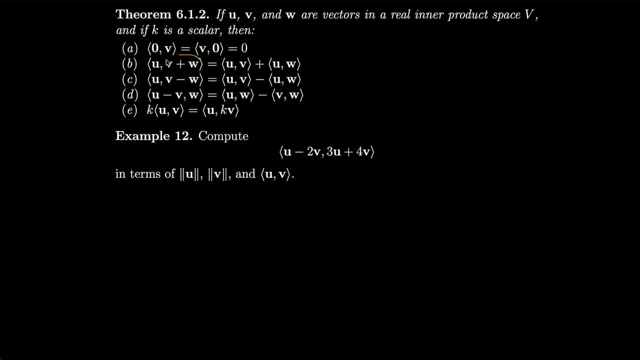 then you're going to get 0.. It turns out you can distribute addition in the second component. That should make sense, because you could always swap these right. You can also distribute subtraction, and you can also distribute subtraction in the first component. 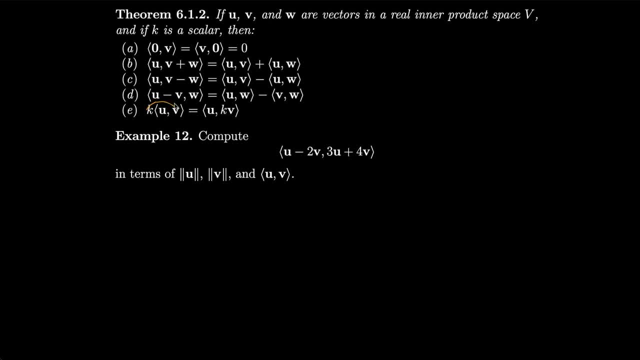 And you can distribute the scalar to either one, so you get all of those for free. As an example, how about we compute u minus 2v, the inner product with 3u plus 4v, in terms of the lengths of u- v and the inner product of u and v? 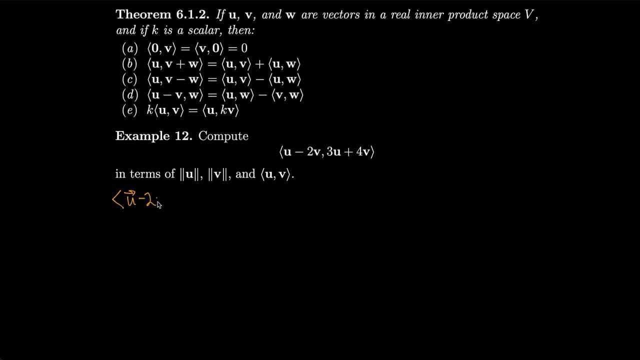 So we'll take u minus 2v, inner product 3v, u plus 4v, that's equal to well. how about we separate off the u, the u by itself? so we'll keep the 3u plus 4v in both. and it was minus 2v, so we'll subtract off.